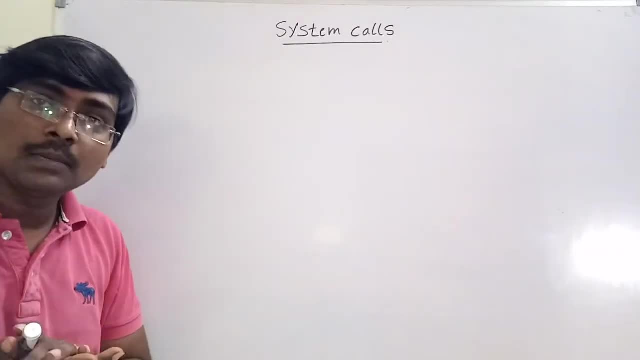 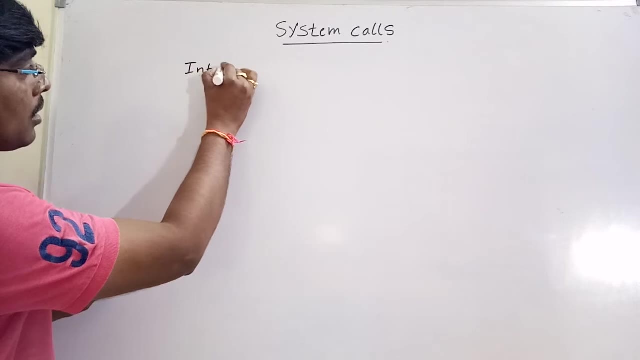 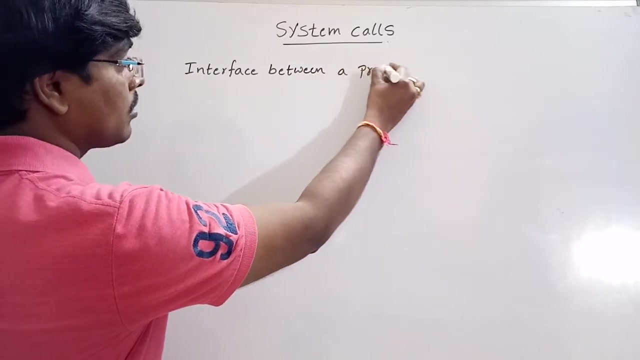 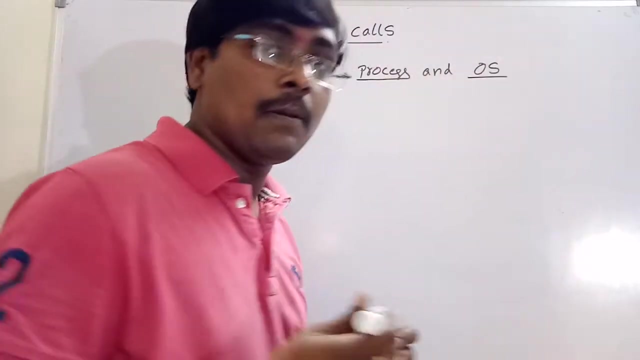 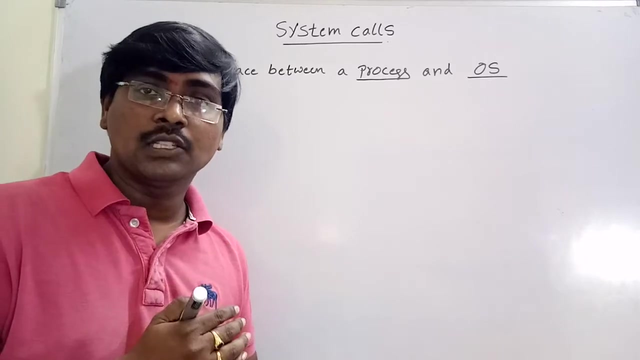 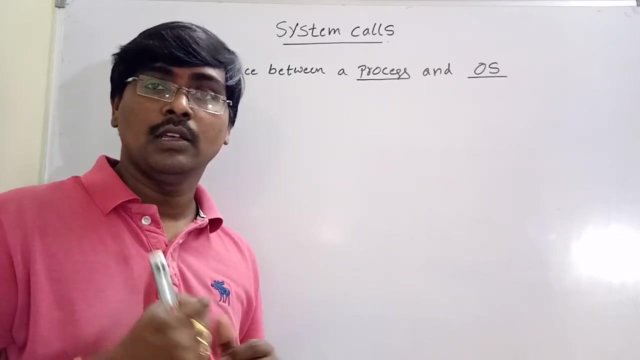 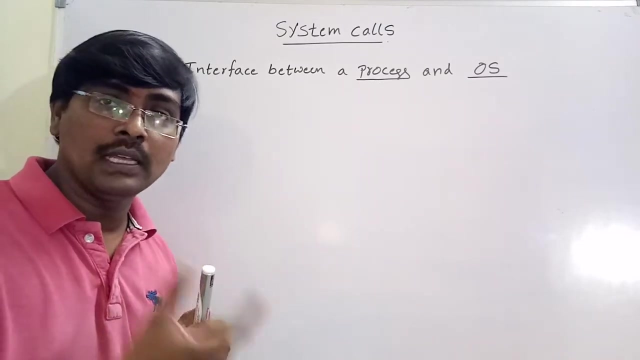 Welcome to our channel. Today we will discuss the concept of system calls. What is a system call? System call is simply an interface between a process and an operating system. System call is an interface between a process and an operating system. Here. what is the meaning of this one? For example, consider a simple program to read data from one file and copy the data into another file. A simple program. What are the operations we are performing? First, you have to open the file. So here, open is a system call. Open is a system call. Read the information from the file. Read the information from the file. 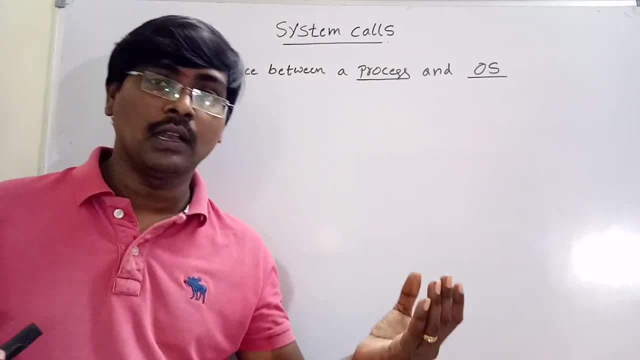 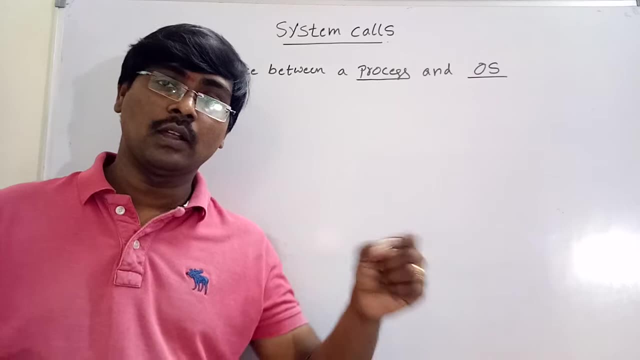 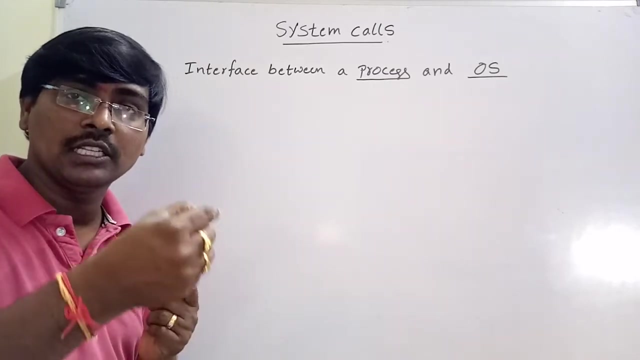 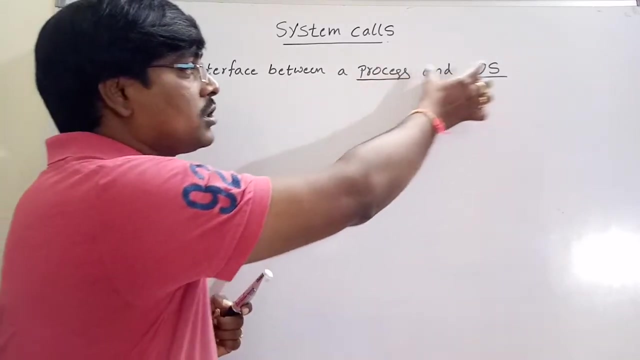 Open is a system call And you have to open the second file and copy the contents from first file to second file. That is, perform right operation and close the first file and close the second file. All these are system calls. That is simply a function that is performed by the particular process. System call is simply an interface between a process and an operating system. We are considering a simple program. Observe even: 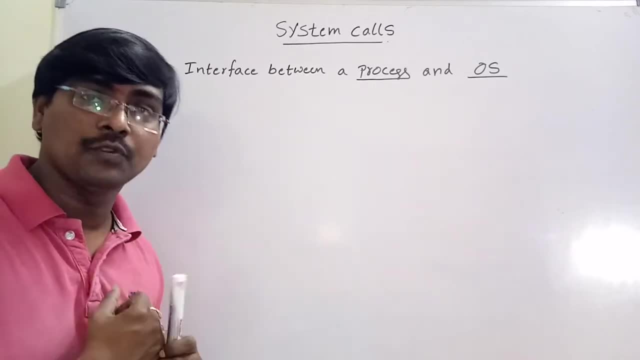 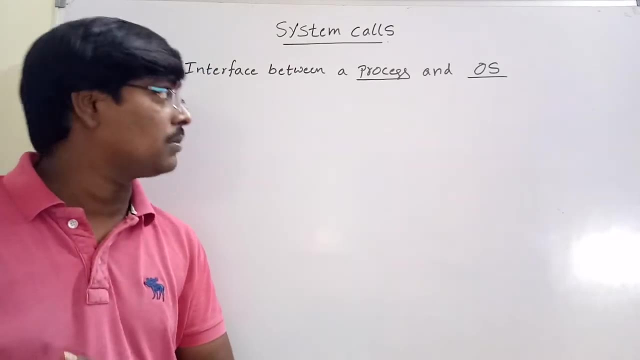 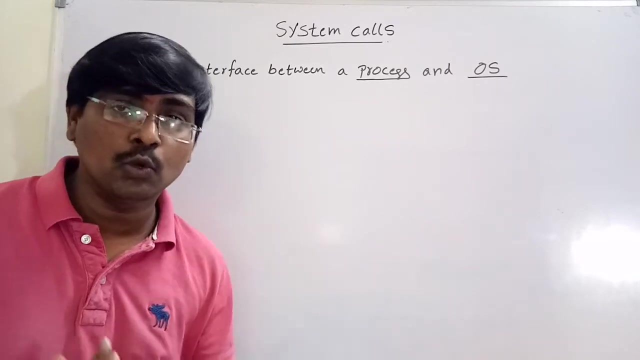 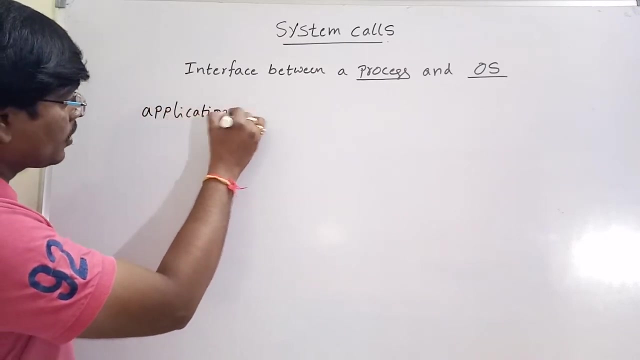 the simple program contains many number of system calls. That is, you execute a simple program. we required many number of system calls. So to overcome that problem, that is, if to call many number of system calls by the user, what the application developers? application developers. application developers. 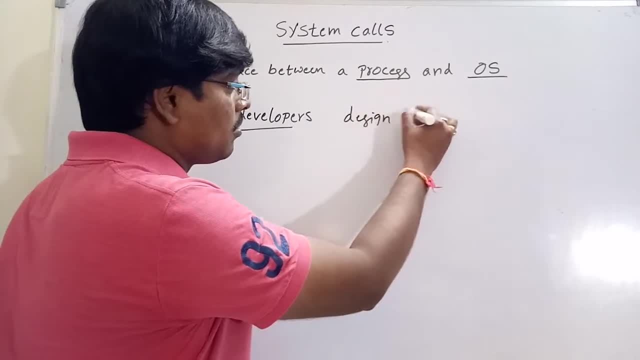 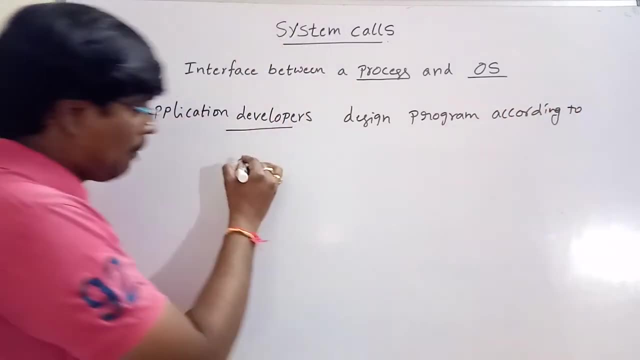 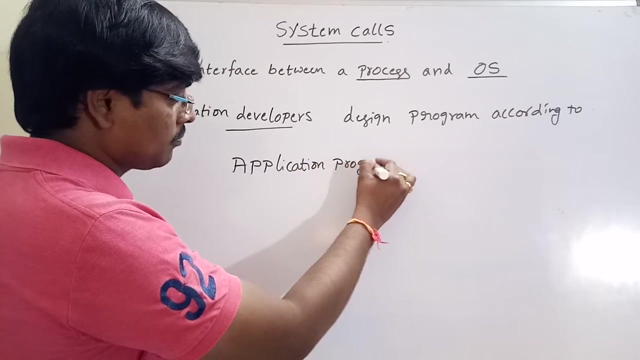 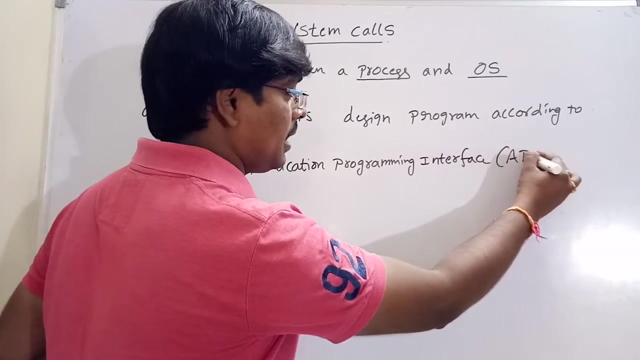 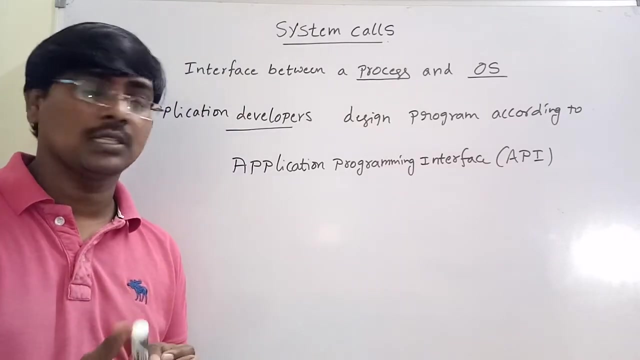 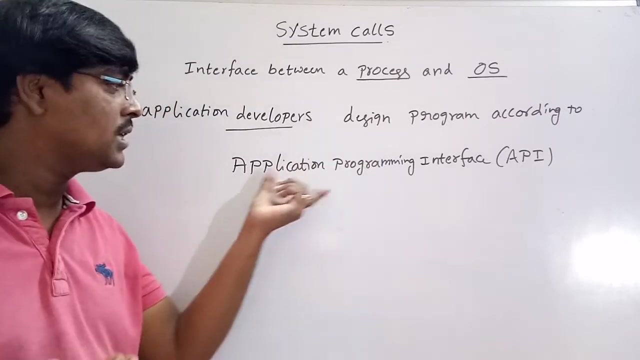 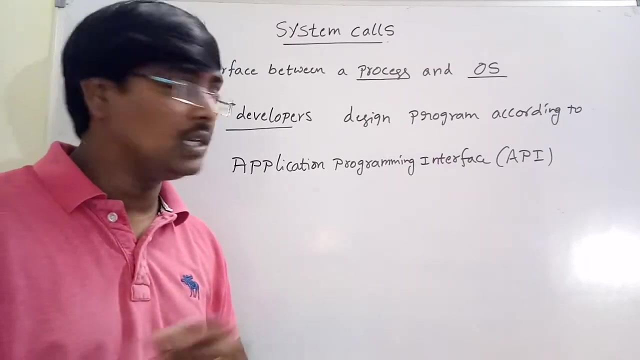 design their programs, design programs according to application programming interface interfaceThat is ABI. That is, for a simple program we have to call many number of system cars. so, for that purpose, what the application developers do? application developers design the programs according to the application programming interface API. what is this API? no question is: what is this API API? 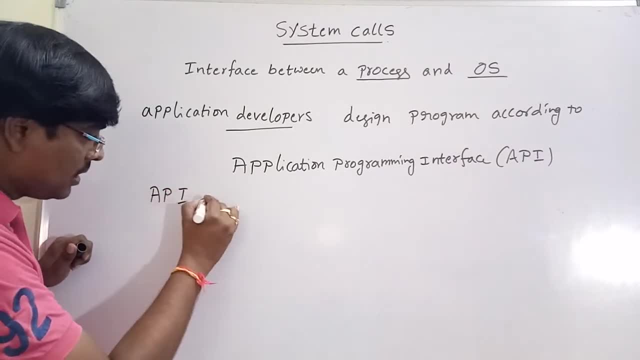 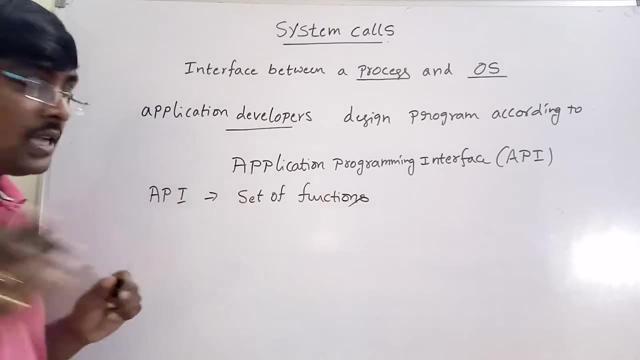 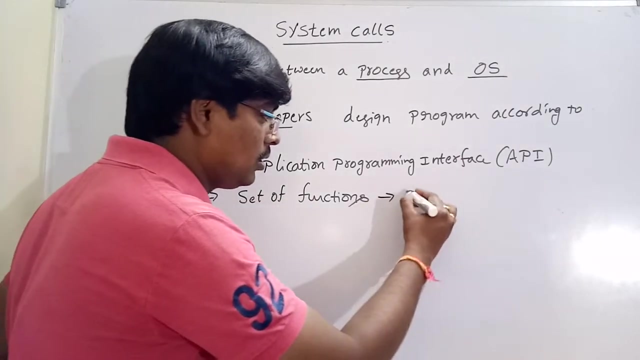 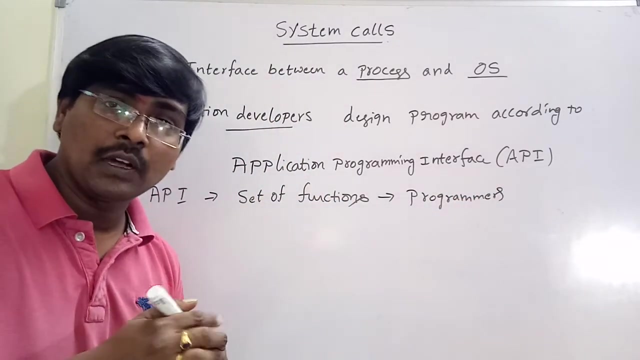 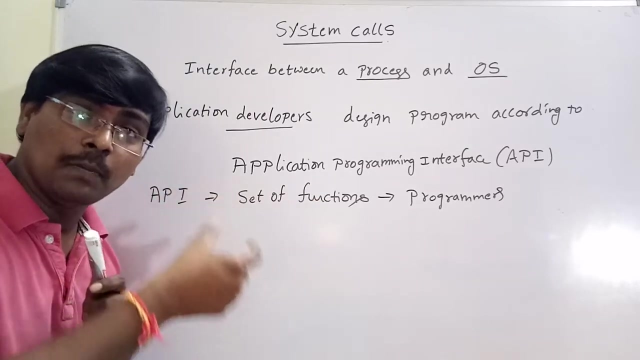 contains simply: API is contains a set of functions. what this API? API contains simply a set of functions, and the functions are available to the programmers. observe: API contains some set of functions and the functions are available to the programmers. along with the functions, the, the parameters are also passed to the function and expect the return type of. 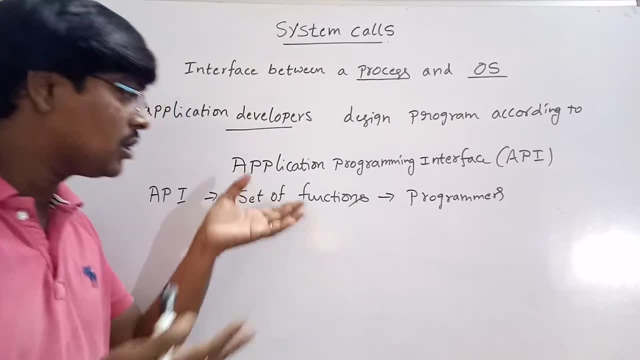 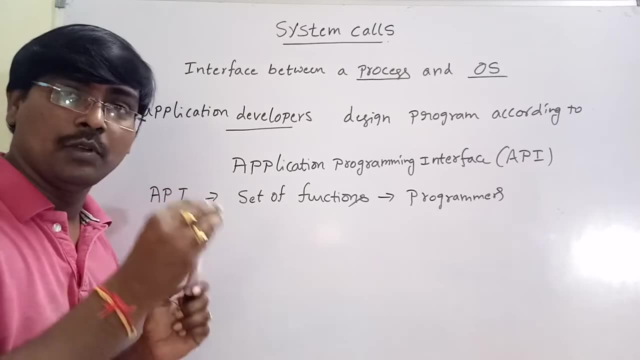 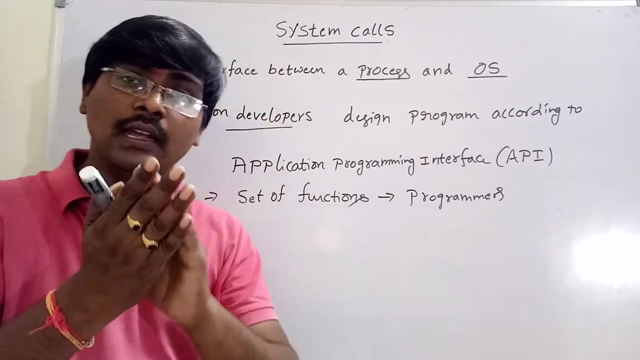 the particular user, that is, which type of information is returned by the user. that information is also present in API, for example. for example, if you are using stack, if you call push operation here, simply we call push, then automatically the entire push operation is performed here. that is a push, is a function. 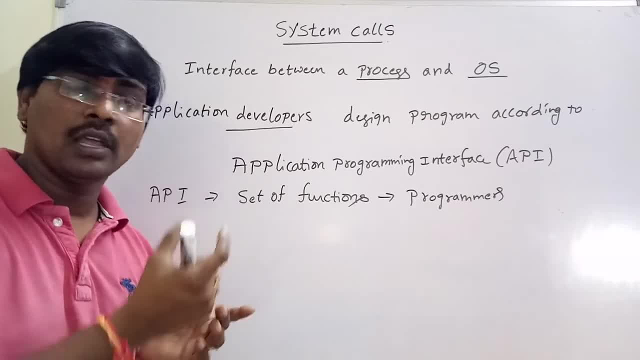 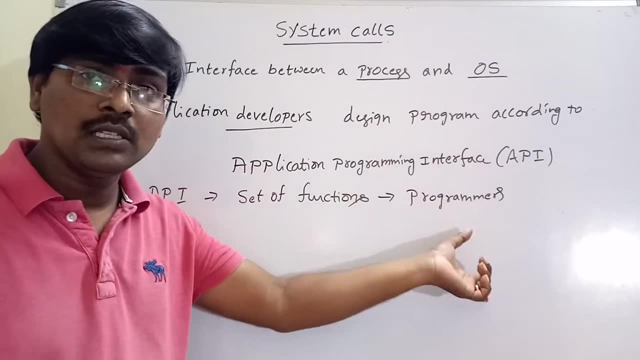 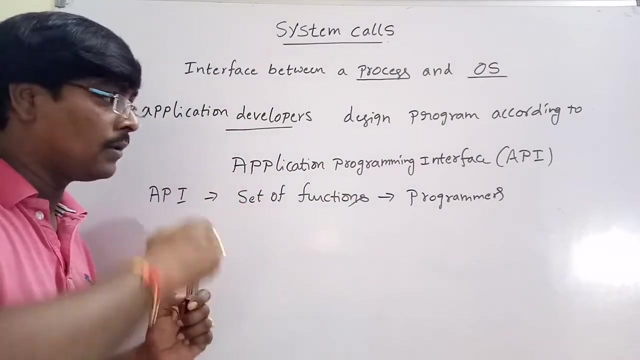 available in stack API. suppose NQ. NQ is a function available in Q API. whenever we are calling that particular Q, that means automatically the functions available in the Q can be utilized if you are called NQ operation. so what are the parameters of NQ by? 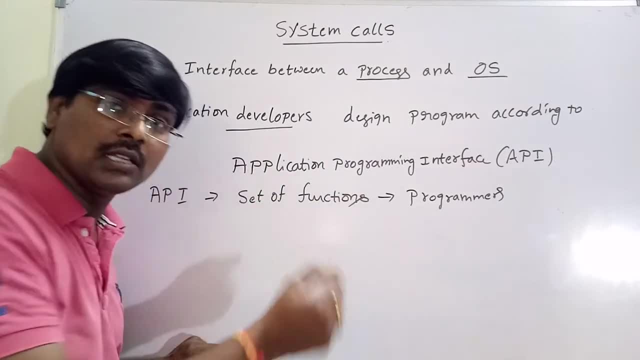 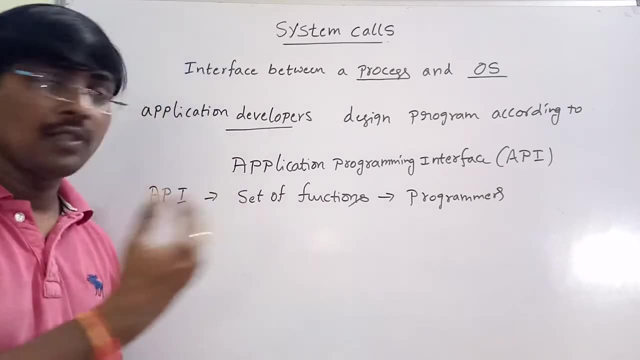 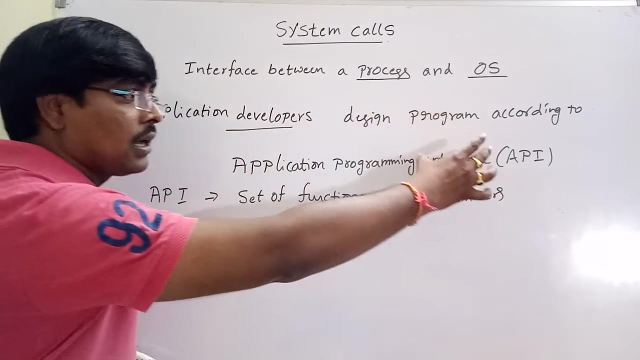 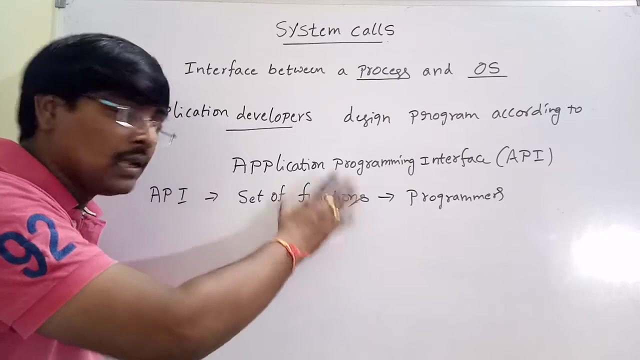 default the parameters are passed to the function. that is for NQ. we have to pass some one parameter. that is the element which want to insert DQ. the element we have to remove. that is simply application programmers develop the programs according to the CPI. now an API is designed. this API contains set of functions and these: 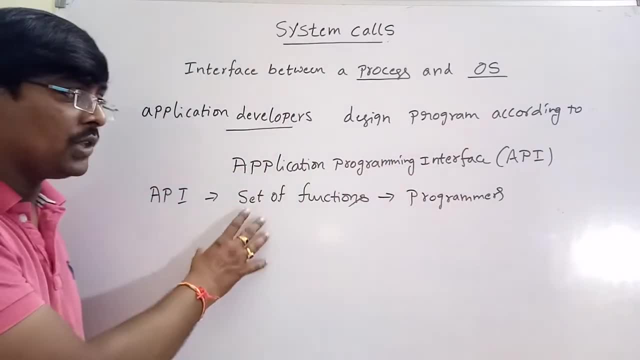 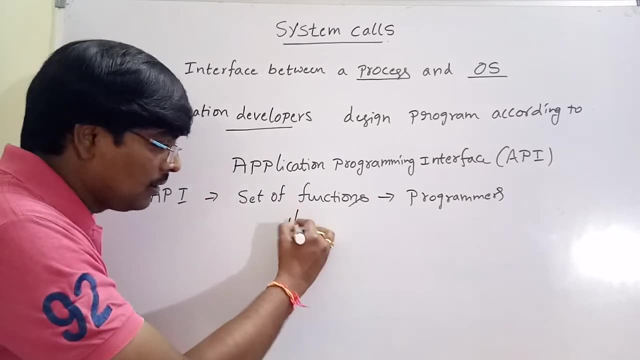 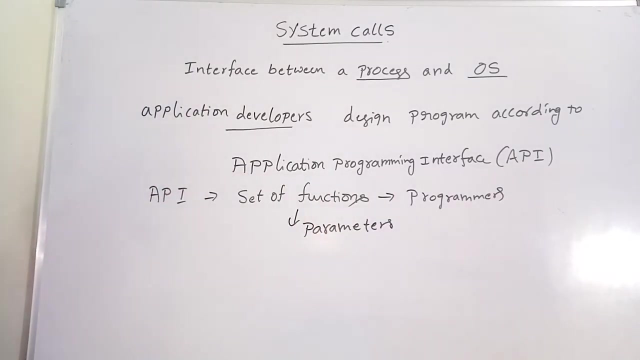 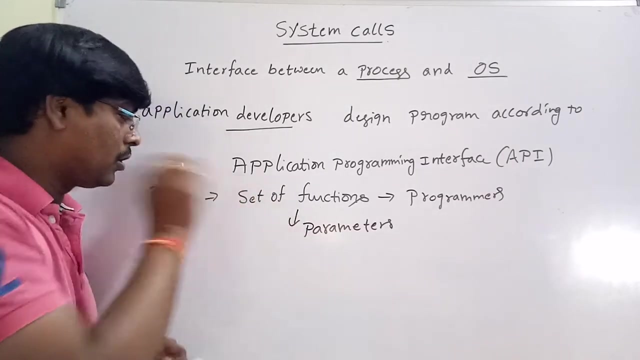 functions are available to the programmers. these functions are available to the programmers and along with the functions, along with the function, they also specify parameters that are possible to the function, parameters that are possible to the function in the return values of the programmer. so what are the return value of the particular programmer? this is the 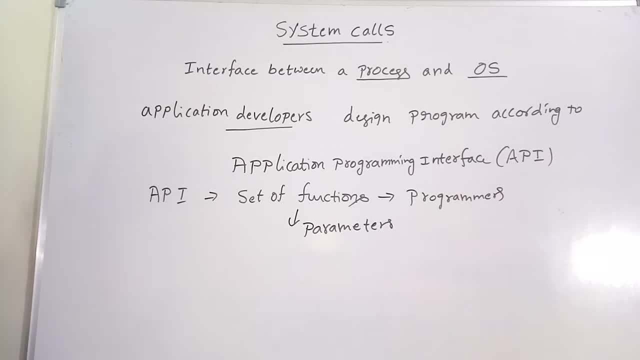 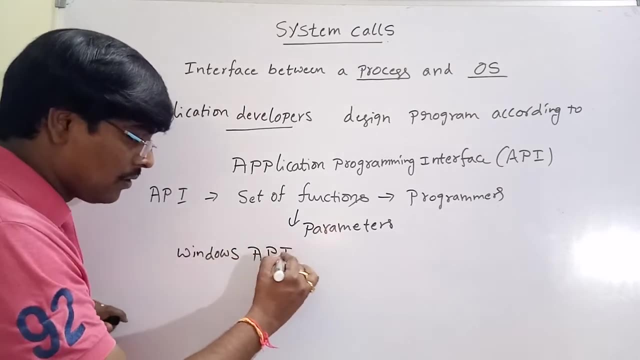 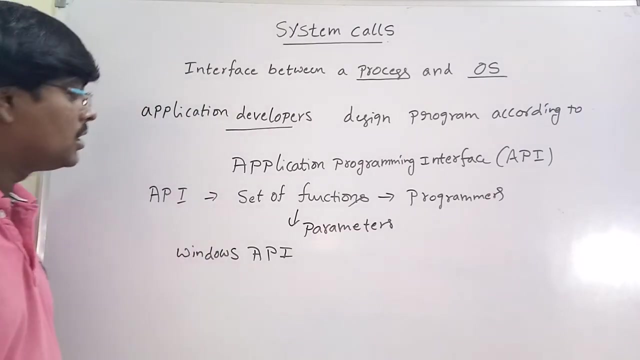 API. okay, this is an API, for example, everyone know. for example, for Windows operating system, Windows API for POSIX, POSIX API for Java virtual API, for Java virtual mission. the API name is Java API. the API name is Java API. okay, once this API is understood, what happens whenever programmer wants to call a function? 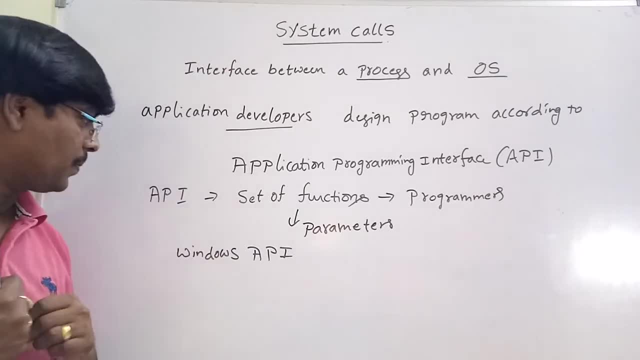 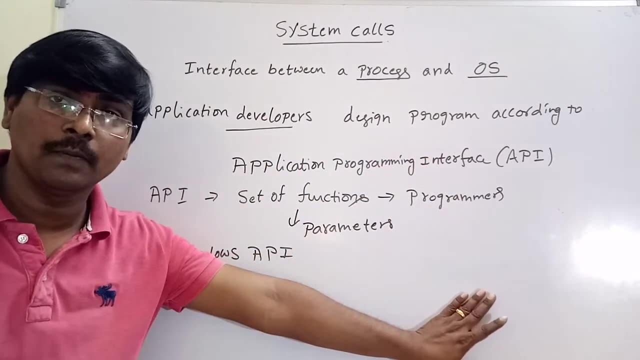 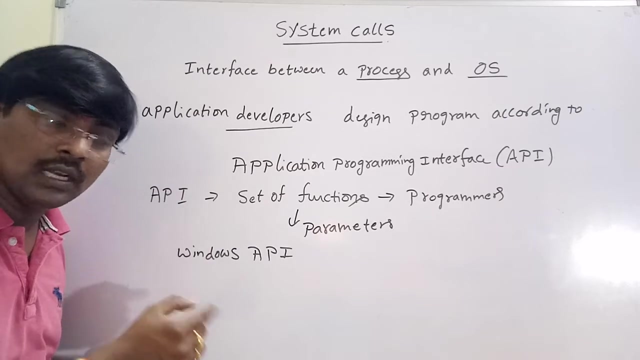 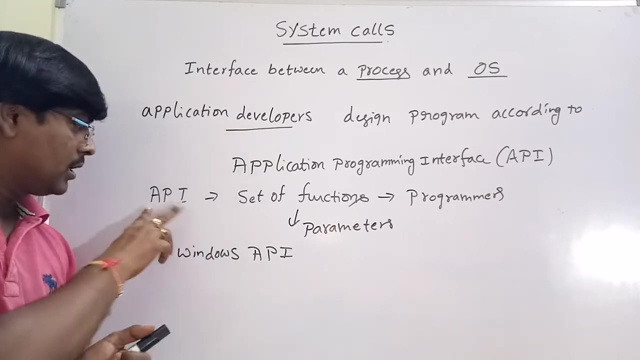 actually it does not call that particular function. suppose the programmer wants to access a particular function, he directly not called the system call. the programmer called the particular API and on behalf and on behalf of the user, the API invokes the particular system call. got it again. I will explain here. the user directly not called any system call. 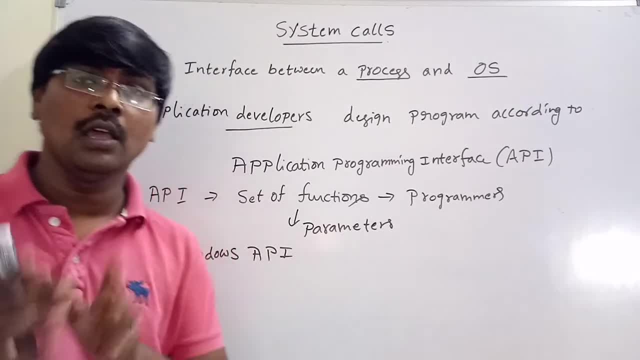 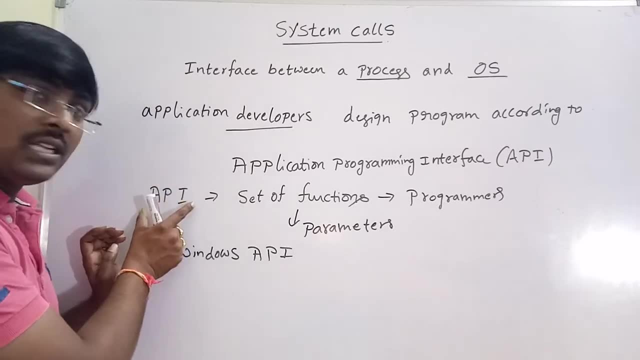 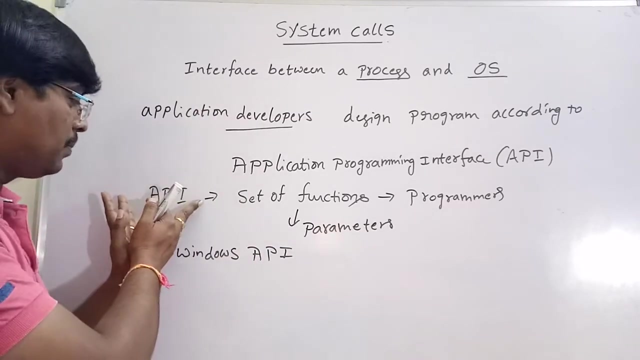 user directly not called any system call. the user can access the API. the user can access the API and this API invokes the particular system called on behalf of the programmer. simply, we are directly not connected to the system call. we are connected to the API and this API connected to the system call. API connected to the system call. 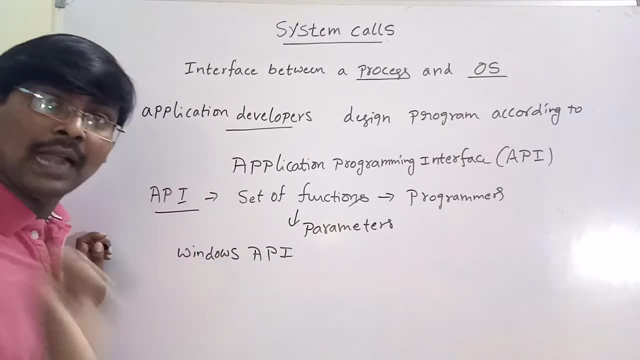 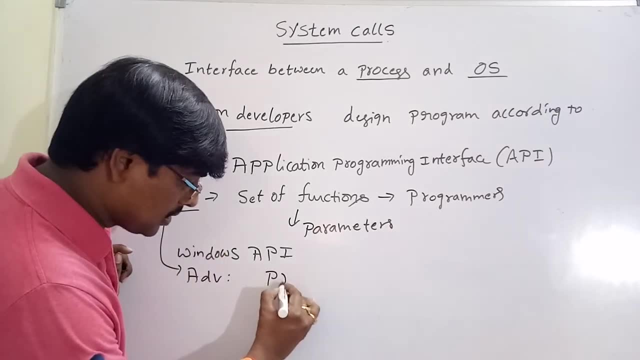 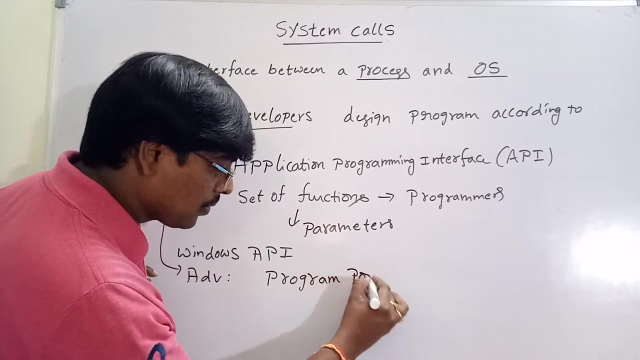 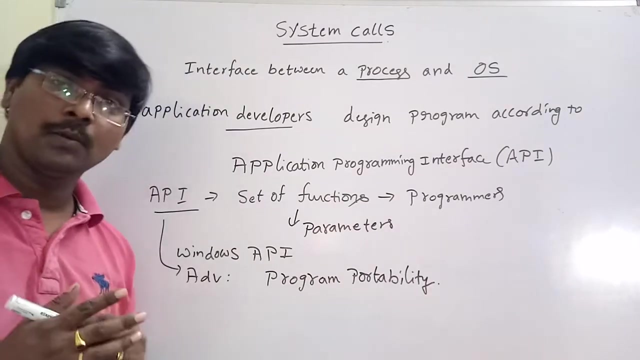 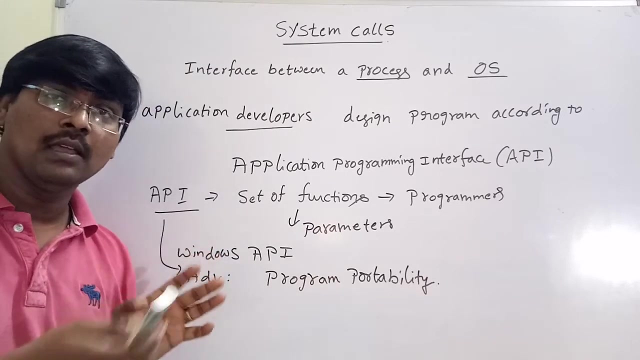 okay, that is API. what is the main advantage of using API? main advantage of using API is, that is, we are designing the programs by using API. main advantage is program portability. what do you mean by portability? program portability, that is, if we design the functions, that is, if we design the program by using API. we 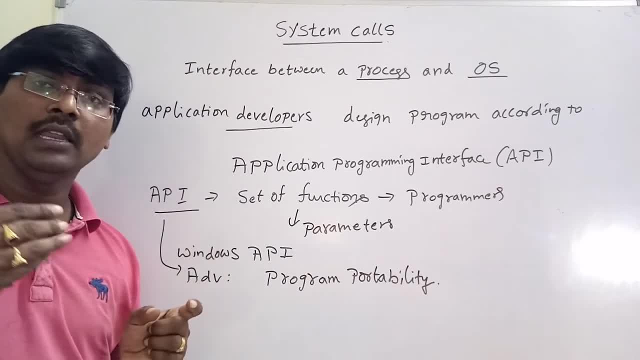 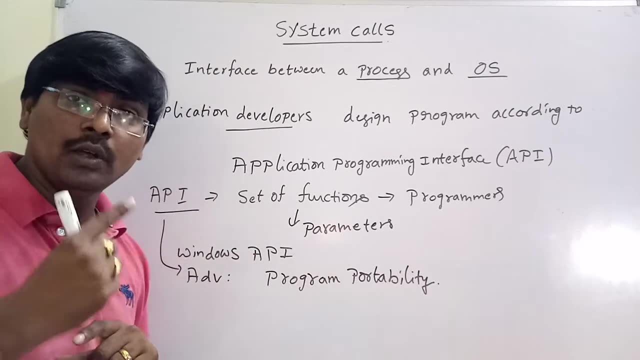 can compile, run and execute the program on any mission, on any mission that supports the same API. that is, again and again, no need to call the system call, simply we call this system call. and again and again, no need to call the system call, simply we call this. 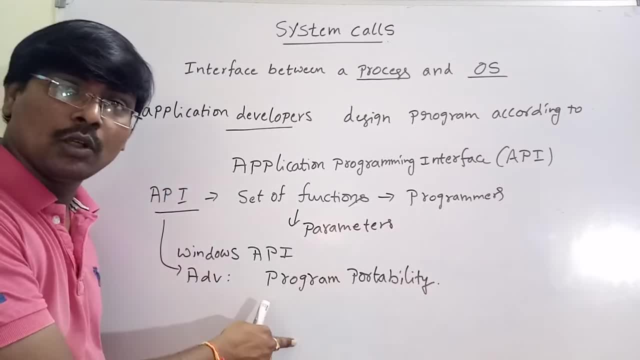 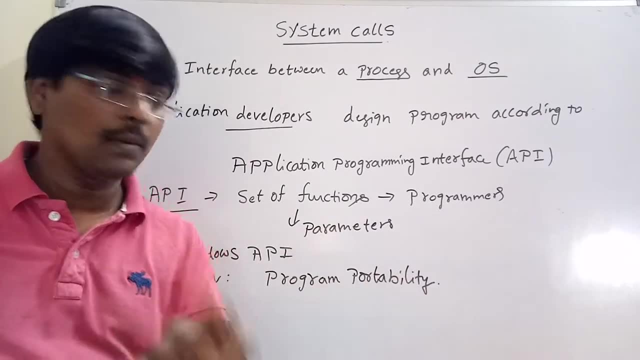 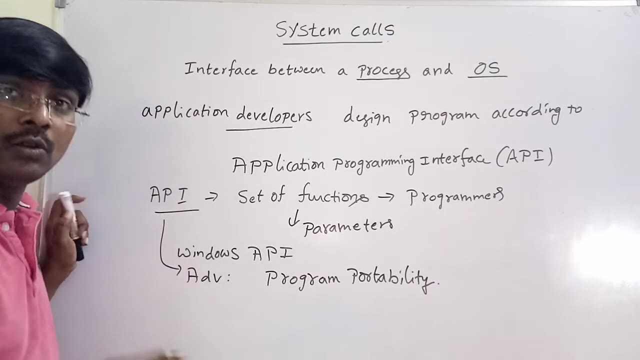 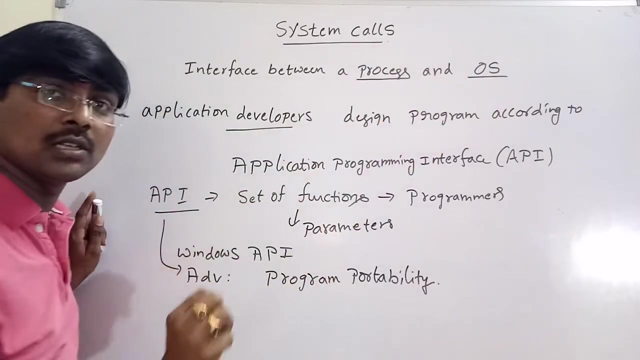 API on any mission, the particular program is executed. okay, program portability means we can run the program on any mission. remember: even that mission supports the same API. the machine supports same API. okay, again within two minutes. what is system call? system call is simply an interface between a process and operating system. that means we are performing some. 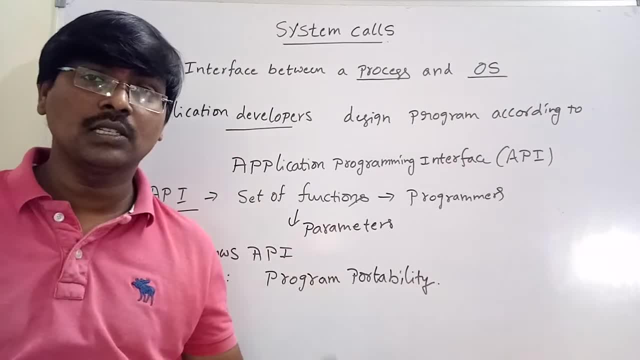 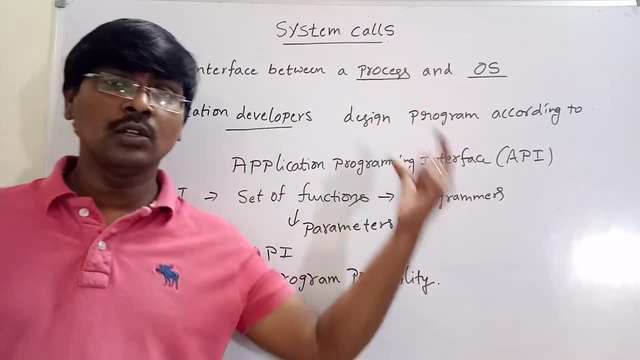 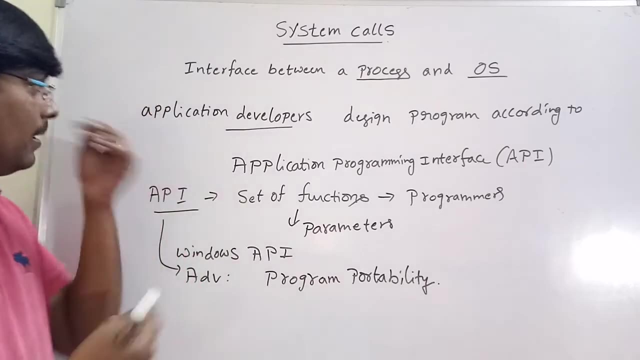 operation. whatever the operation we are performing, that is a system call. suppose I am open on my computer, click on my computer, so that is a system call. close, close is a system call. read, read is a system call. every operation we are performing is a system call. okay, so generally for a simple program, also many. 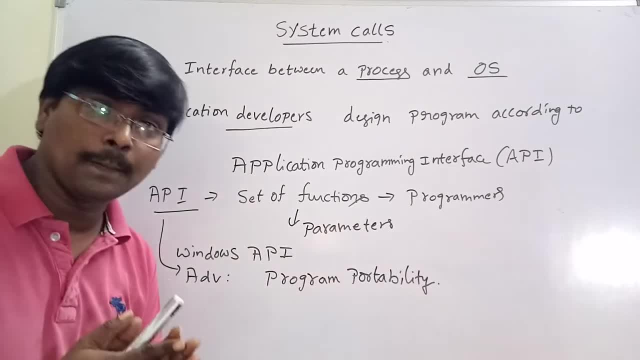 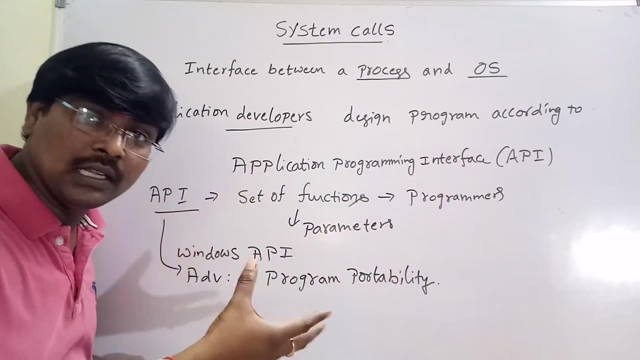 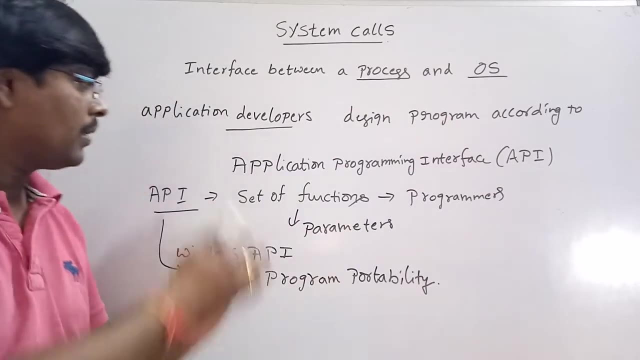 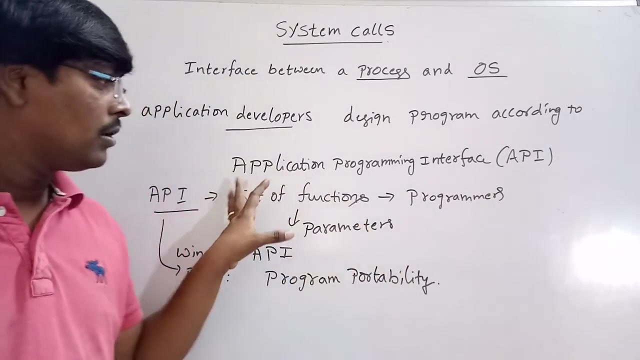 number of system calls have to be executed. for that purpose, application developers design the programs according to an API. that is, an API is designed according to API. application developers design the program. now, what is an API? API is simply a set of functions, that is, simply our predefined functions, set of functions available to the programmers, and remember, along with the function by API, each function also contains the parameters that are passed to the function and the return value of the programmers. the parameters and the return value of the programmer. okay, one of the main advantages in API: how the functions are called, the user do not directly interact. 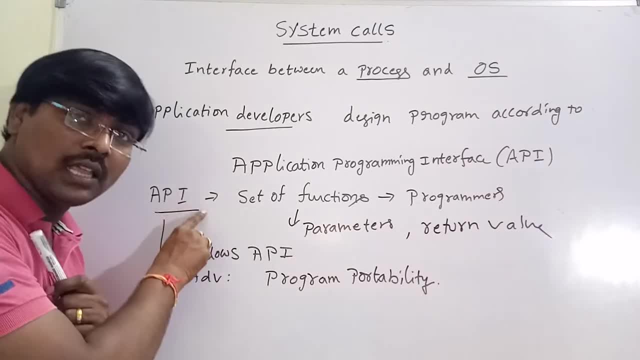 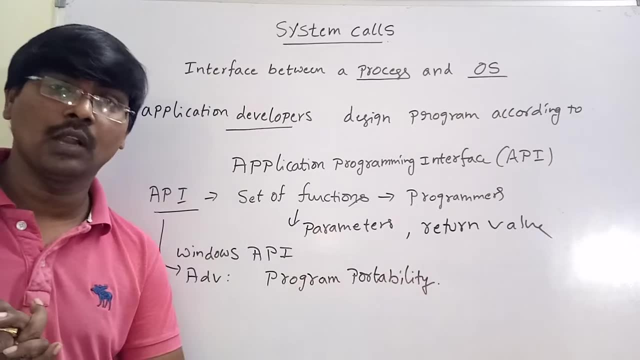 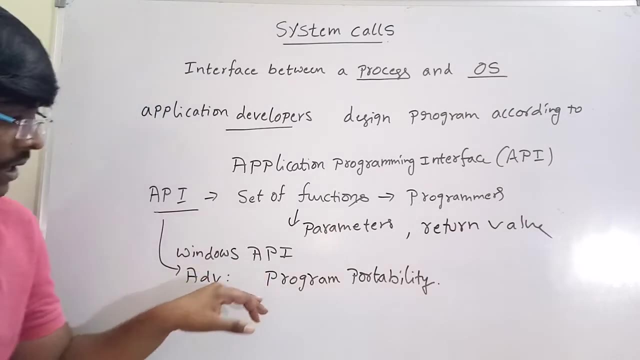 with the system call. the user calls the API and the API invokes the required system call on behalf of the view programmer, on behalf of the programmer. API call the system call. finally, the main advantage of API is program portability. main advantage is program portability. what do you mean by? 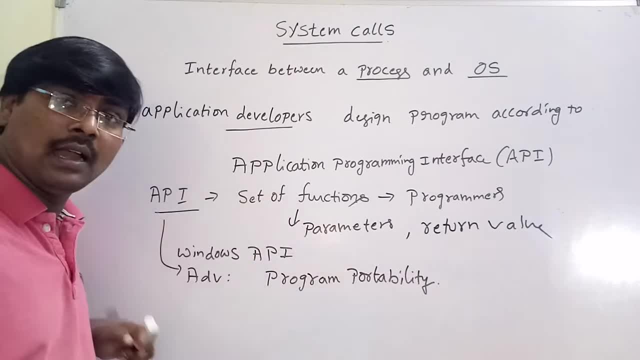 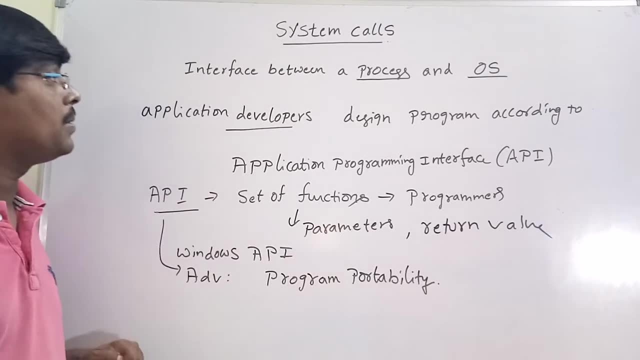 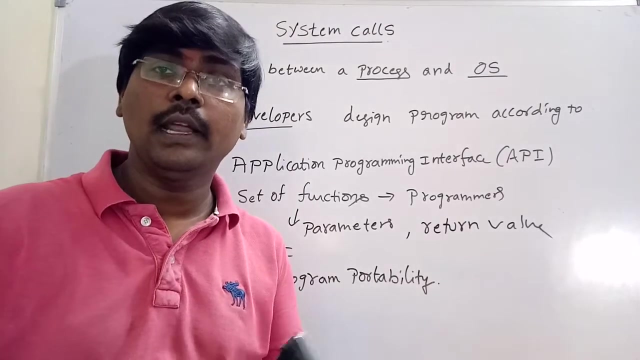 this program. portability: this program can run on any mission, execute on any mission that supports the same API. that supports the same API. okay, this is an API now for every program generally, for most of the programming languages. for most of the programming languages. the runtime support system for most of the programming languages. 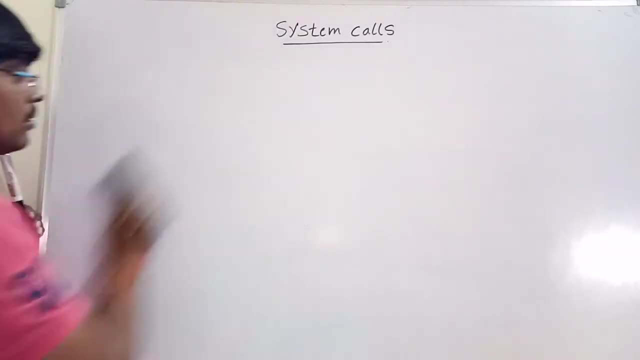 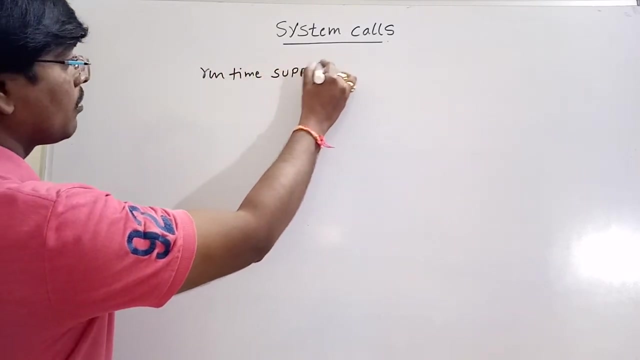 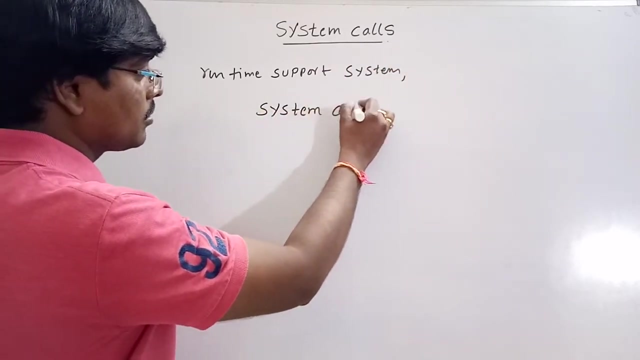 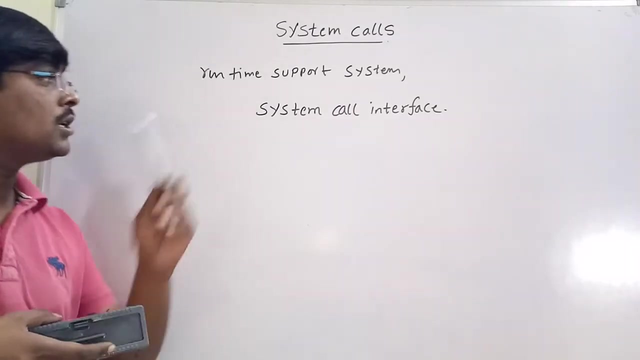 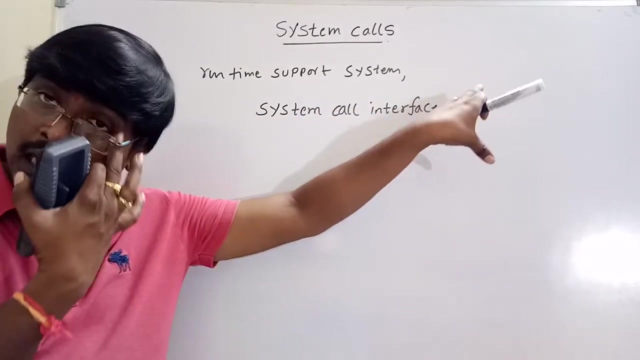 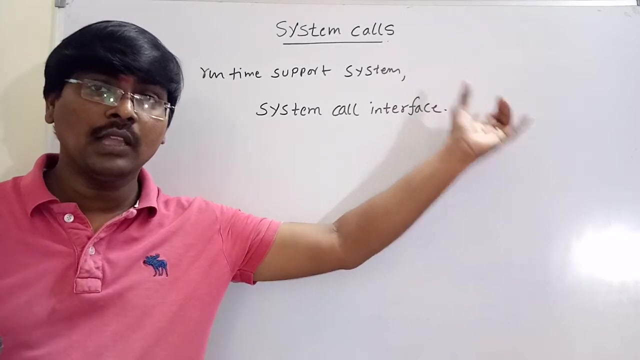 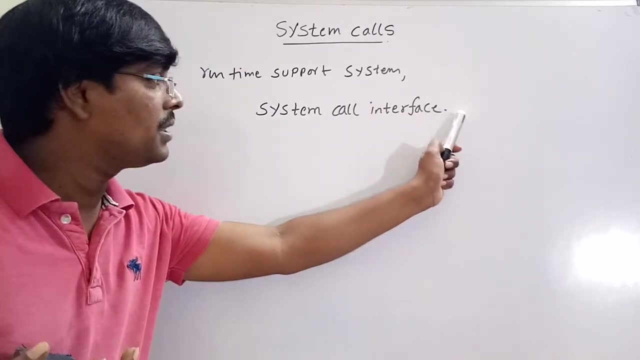 the runtime support system provides system call interface for most of the programming languages. the runtime system supports system call interface. this is system call interface. provides a link to the system cause. the system call interface provides a link to the system call for the operating system. link to the system call that made available by the operating system, available by the. 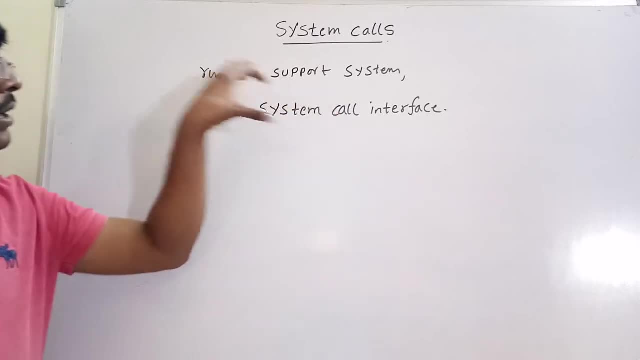 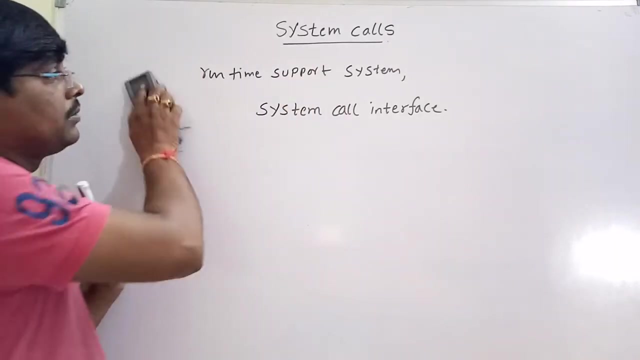 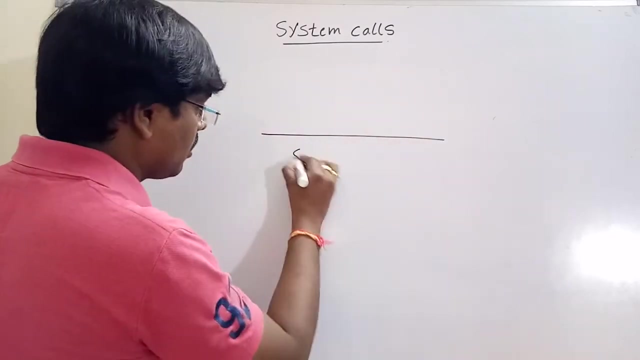 operating system. okay, so simply, every programming language. you have to define a system call interface and this system call interface provides as a link to the, as a link to the operating system, that is system call. now consider an example how the system call interface can work. suppose: system call interface. 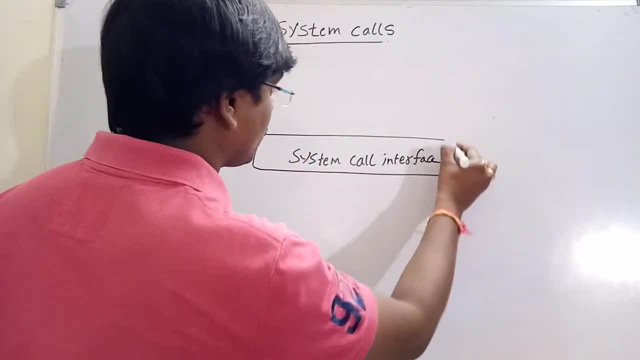 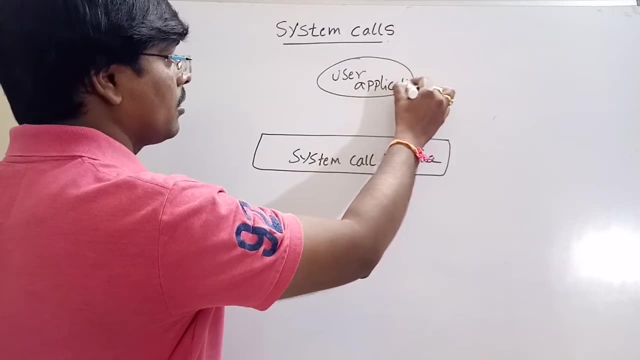 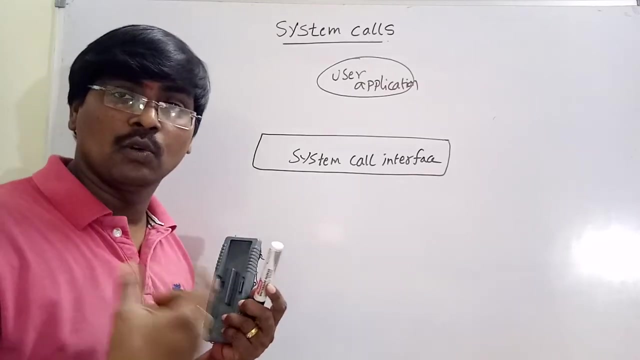 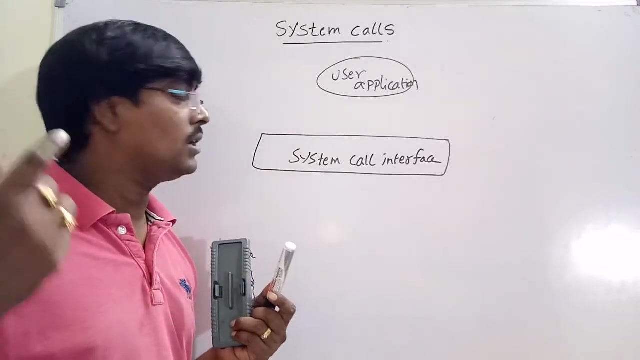 this is some user application. this is some user application. we have two types of modes. one is the user mode, second one is kernel mode. user mode, that is, user operations are performed in user mode. kernel mode is the part of the operating system that is operating system. services are that is. 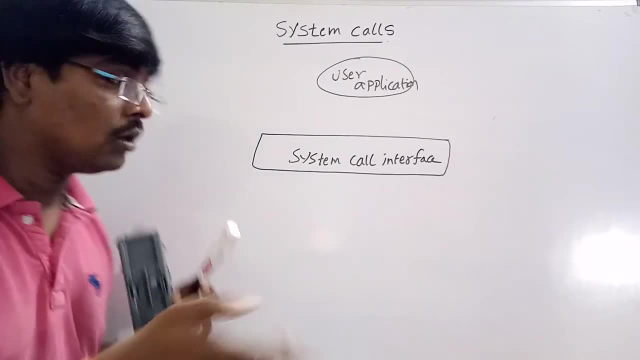 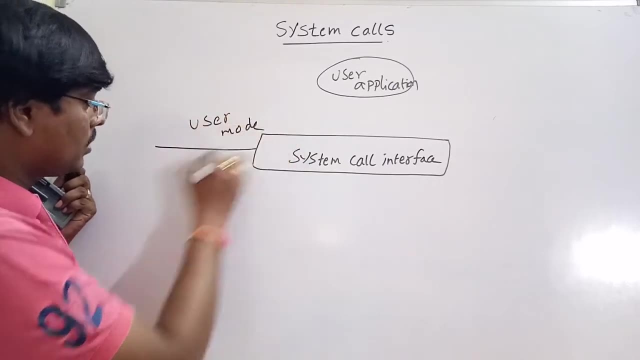 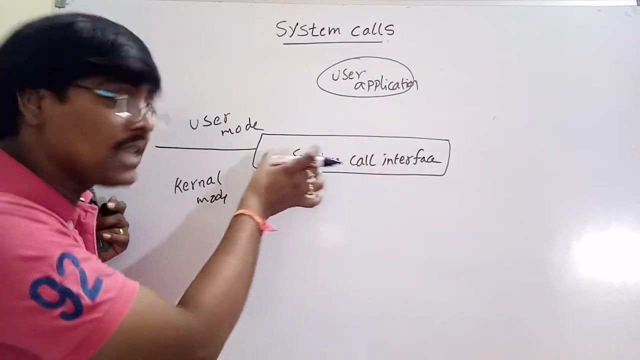 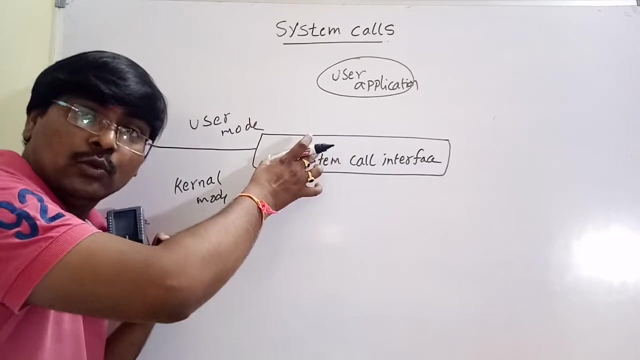 operating system activities are performed in kernel mode. now, this system call interface this one, see this one. this is user mode, this is kernel mode. I think you got the point, that is, this system call interface, access and interface to the this user mode in the kernel mode, that is, by using this interface, by using this interface. 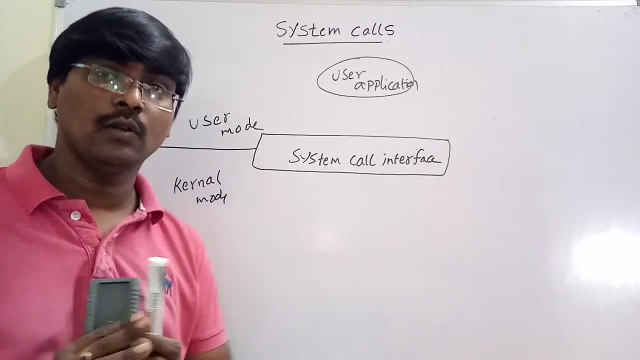 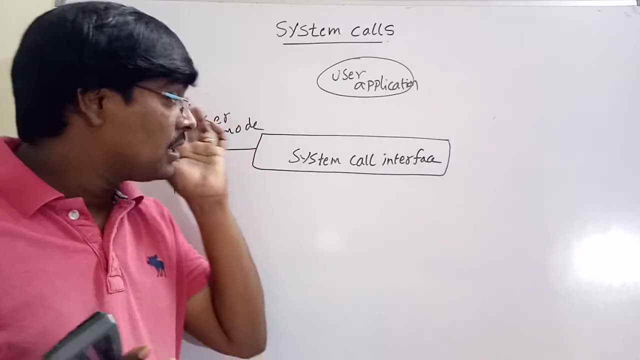 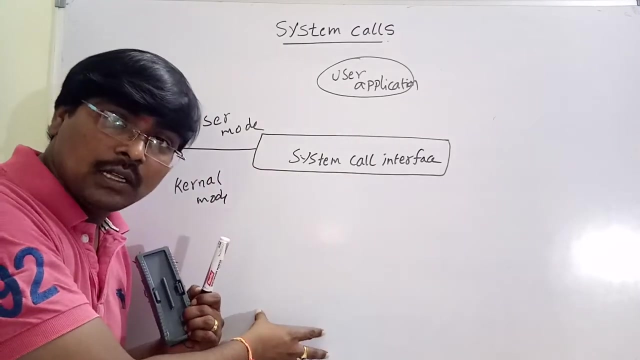 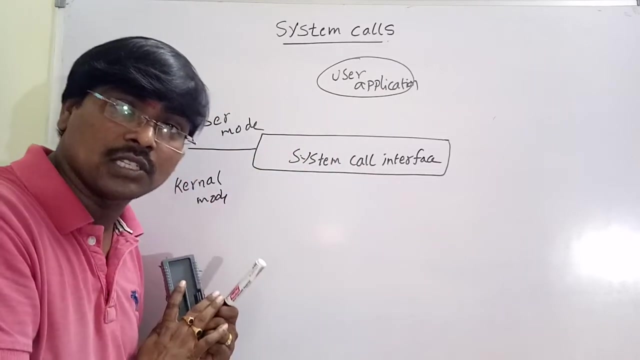 we can access the particular system call. ok now, before going to this example, I will explain one more point about system call interface. each system call is assigned a number. remember, generally we have many number of system calls. all the system calls are placed in api, that is, for all the system calls are placed in system. 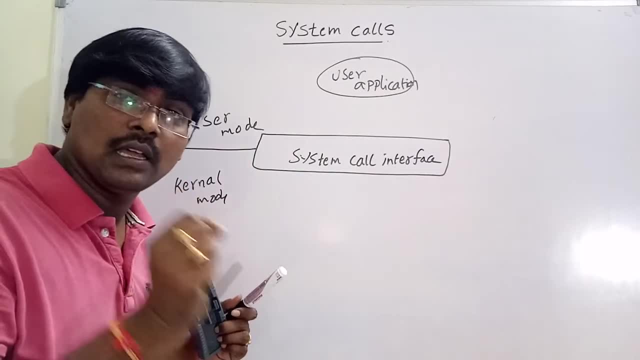 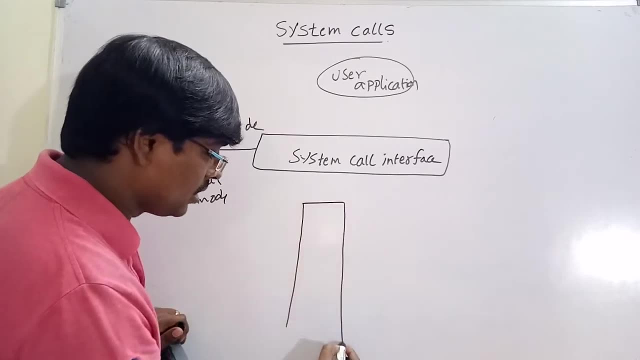 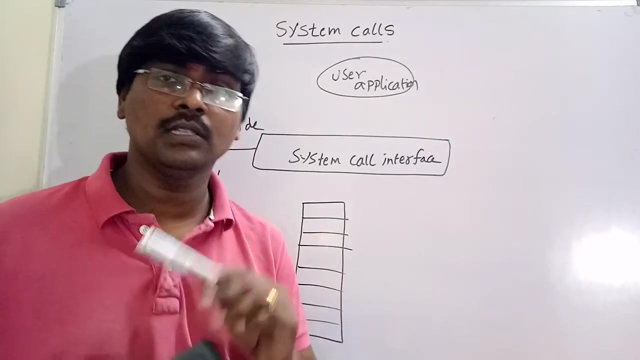 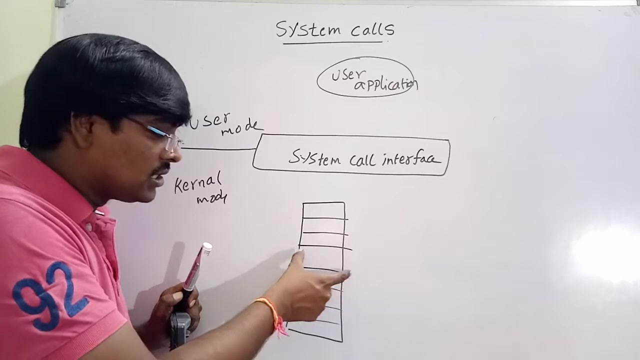 call interface. each system call is has a number, has a number, okay, and all the system calls are placed in a table in this fashion. remember, we have many number of system calls. i am assigning each system call with a number and all the system calls are maintained in a table. this table is: 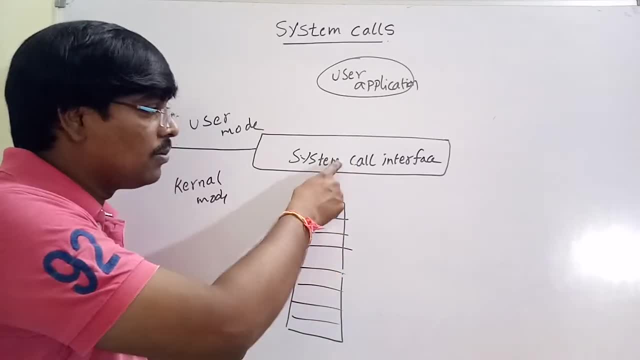 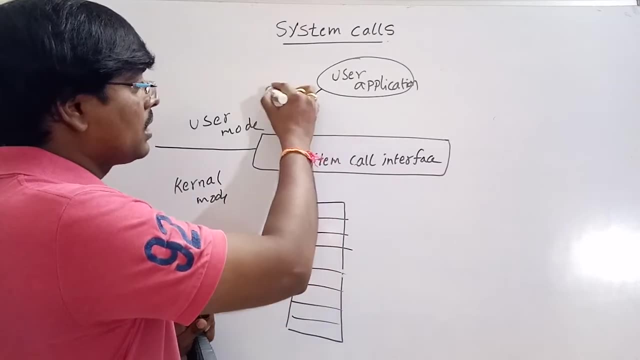 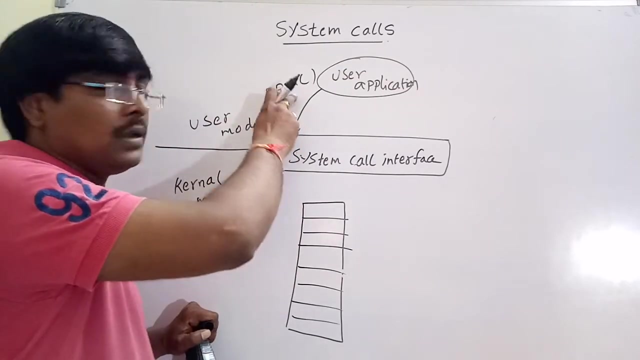 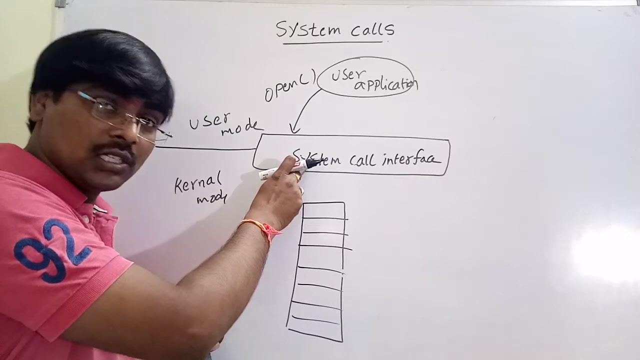 maintained by this system call interface. this table is maintained by system call interface. okay, now what happens? for example, user wants an application open off. user required open off function whenever he required open. then what to do? he calls the system call open. so he directly, not calls simply. he move to the system call interface and this system call interface check the function. 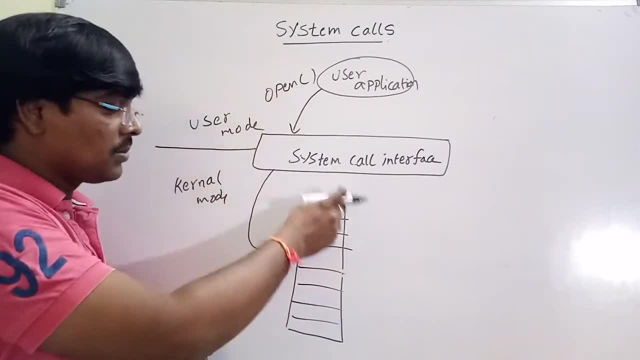 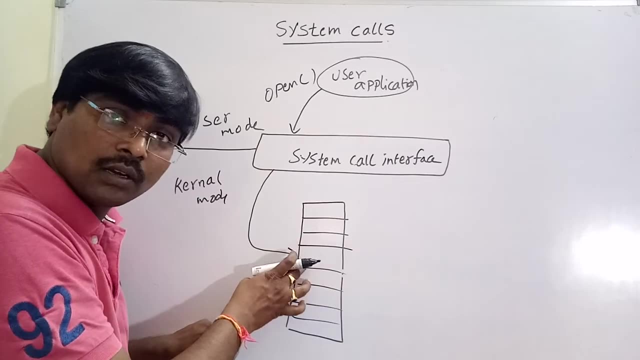 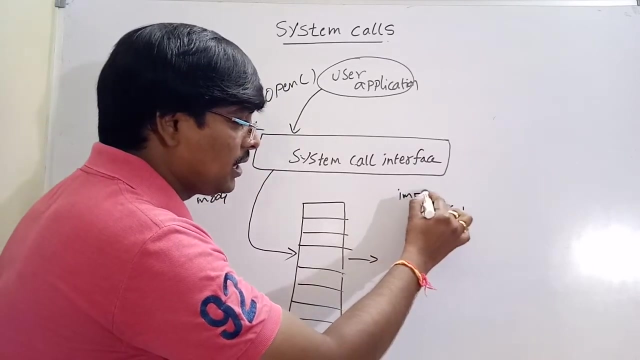 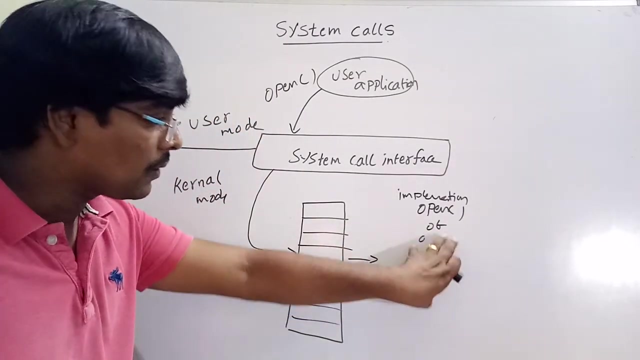 open in the table. okay, each and every system call has number. this is a table of all the system calls. in this table, the open system call is checked once the open is available. for example, this is open, the implementation of open is performed. implementation of open is performed and finally return. 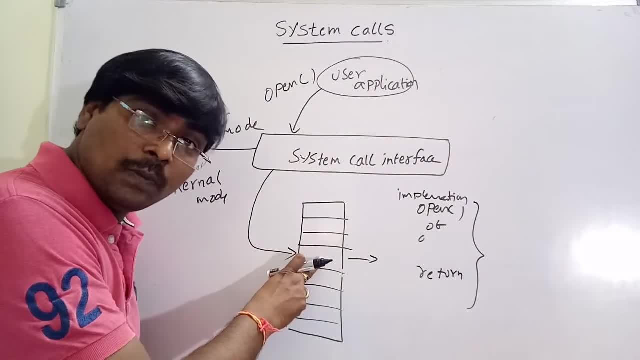 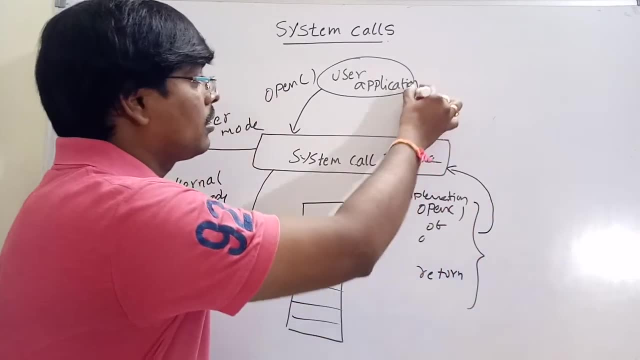 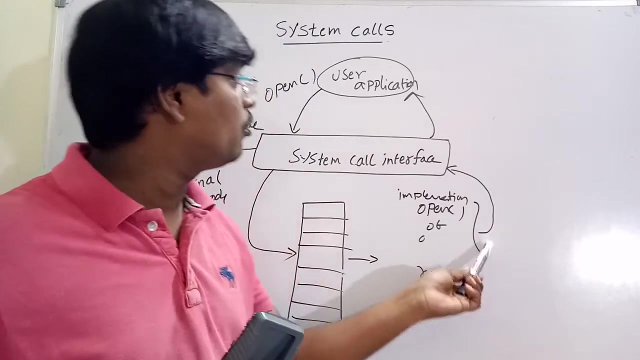 this is happened whenever open function is available, open system call is available, the implementation is executed here and simply it returns the final output. that is written, the concept, that is written, the value of the open to the user application to the user application. okay, this is system call interface. 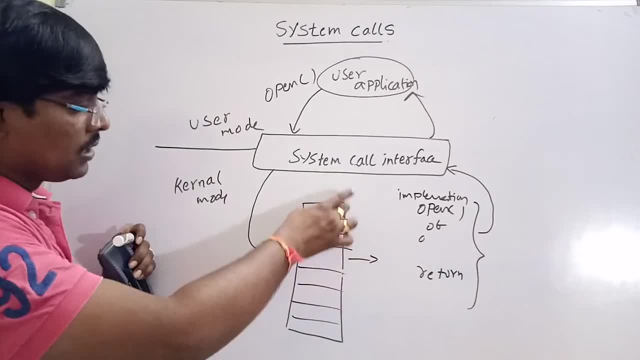 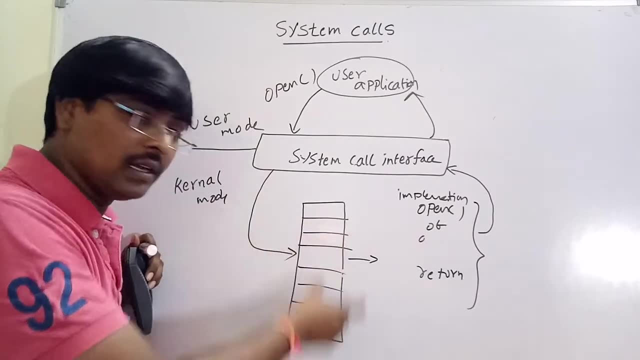 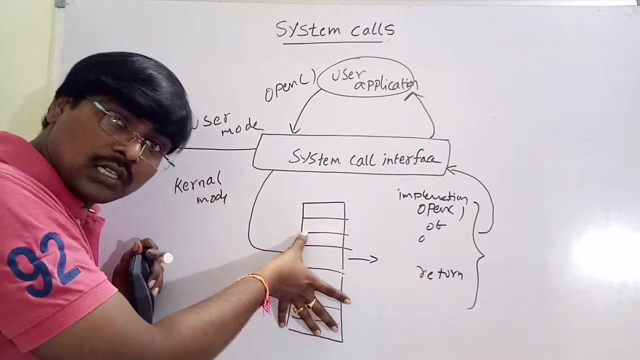 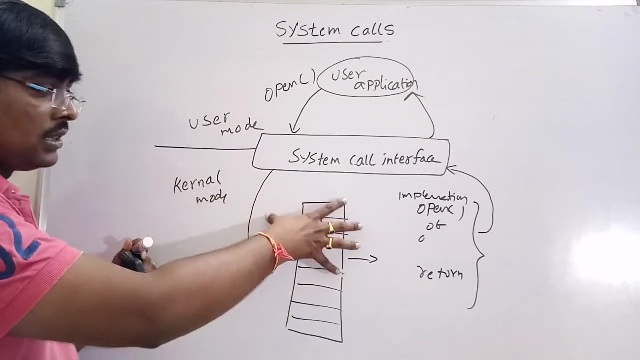 system called interface. okay, in it out simply system call. interface maintains all the system calls and each system call is is numbered. that is, all the system calls are numbered and arranged in the table. whenever we required a function, we check for that particular system call and perform implementation and written the result to the particular user application. this entire. 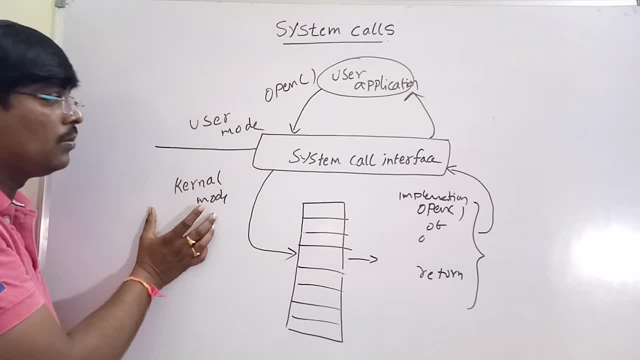 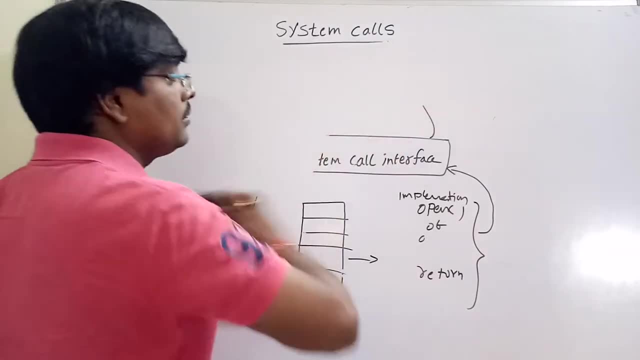 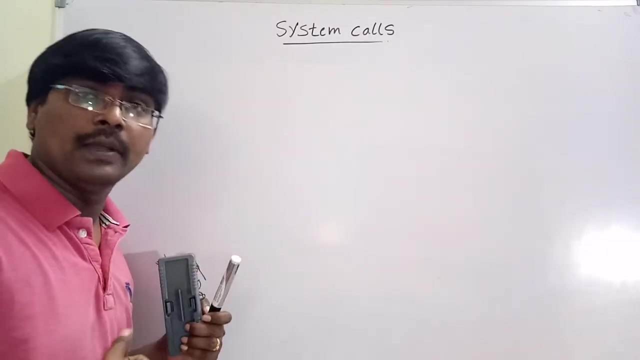 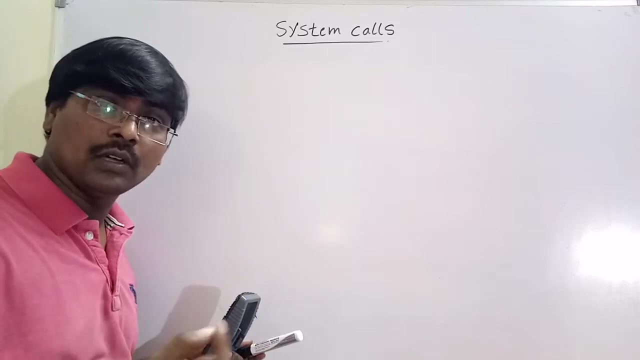 operation is performed in the operating system side, that is, in kernel mode. this is user implementation requirement. that is in user mode. that is in user mode, okay. and finally you can pass the parameters to the operating system to perform operation. that is, we call a function. whenever we call a function, we already said that we have to 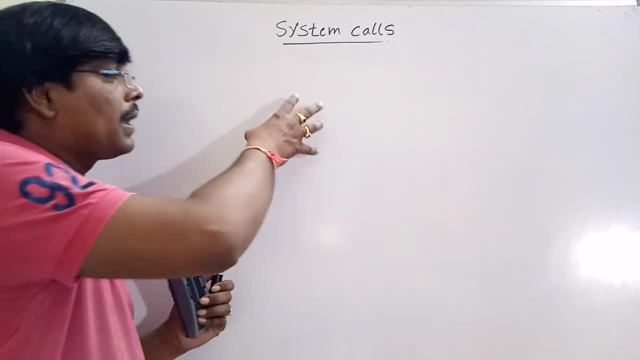 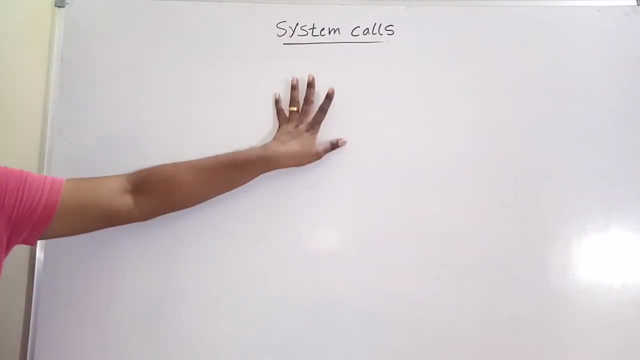 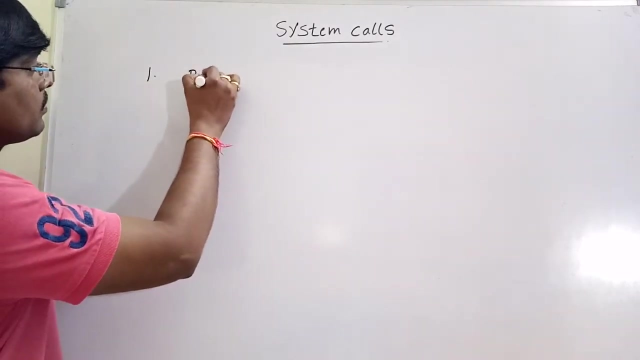 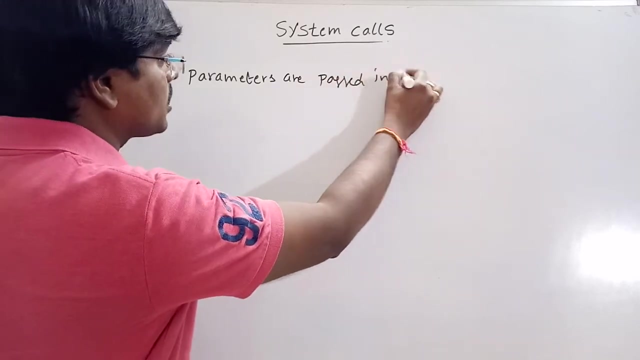 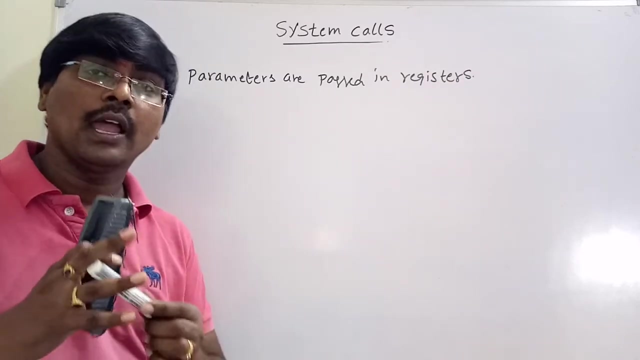 pass the parameters to the function also. so the parameters are passed to the function in three ways. okay, you got it. the parameters are positive. positive in three ways. one is: parameters are positive in registers. parameters are positive registers. for example, I have five parameters, so I am using five registers each register. 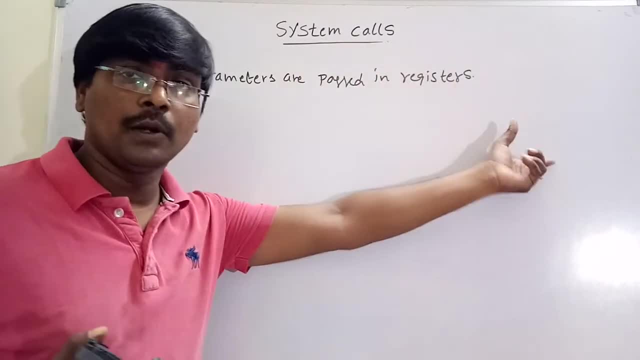 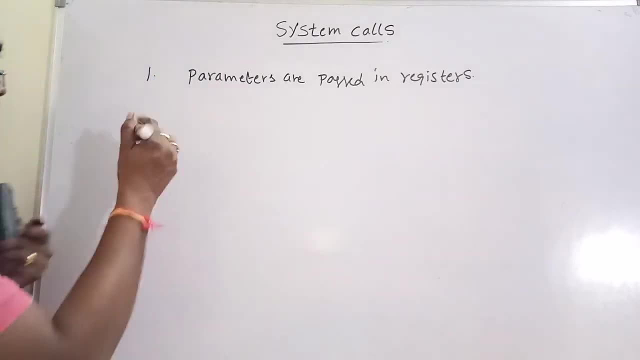 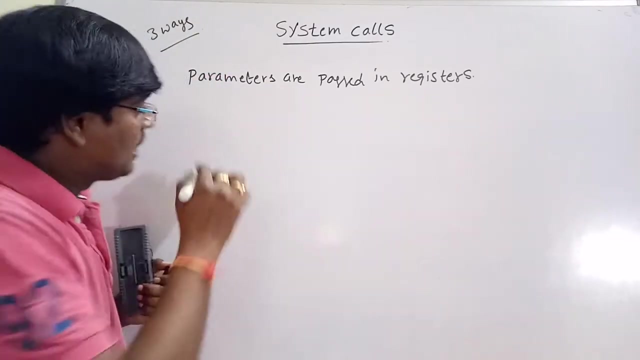 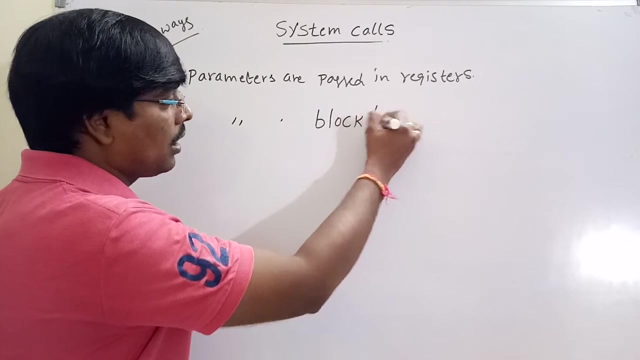 contains one parameter and all those are positive to the particular operating system. parameters are positive to the operating system. second work technique is we have three ways how the parameters are positive to the operating system. second one is the parameters are. the parameters are placed as a block, a table of memory block or table of. 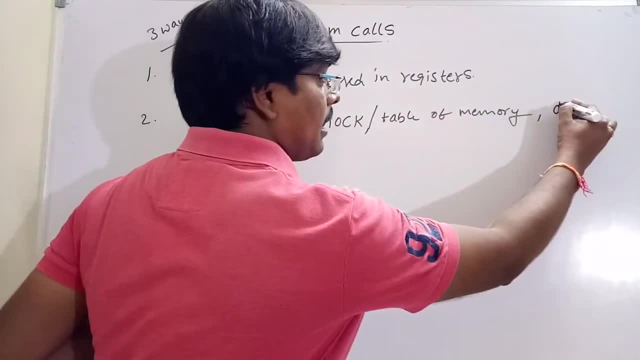 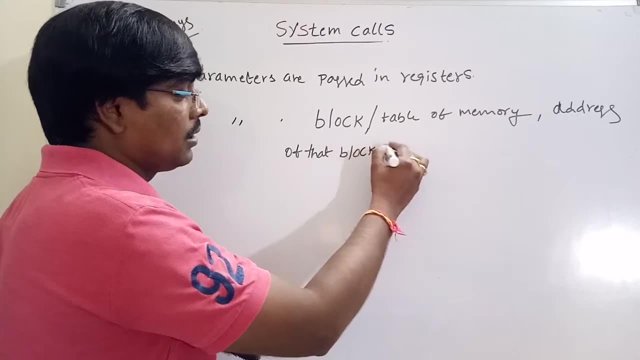 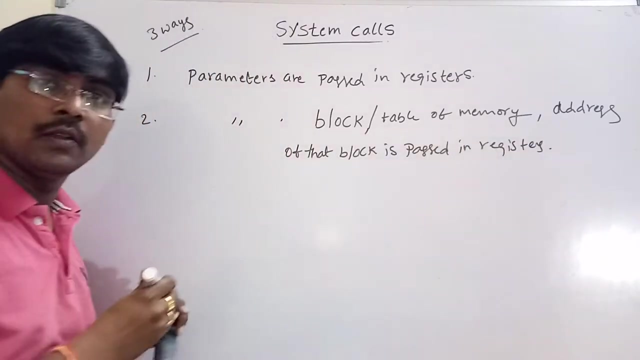 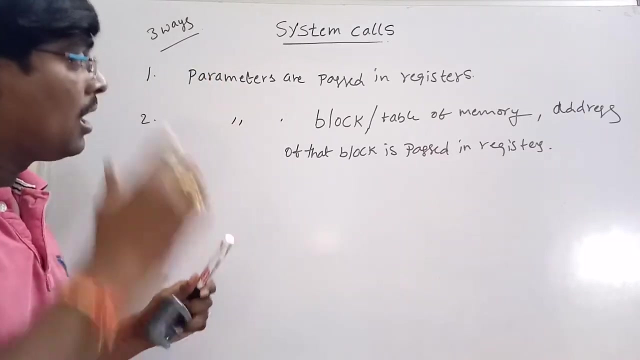 the memory and the address of that particular block. the address of that block is passed in registers, So you got the difference. In the first case, all the parameters are passed as individual registers. In the second case, all the parameters are placed in a block of memory or in a table of memory. 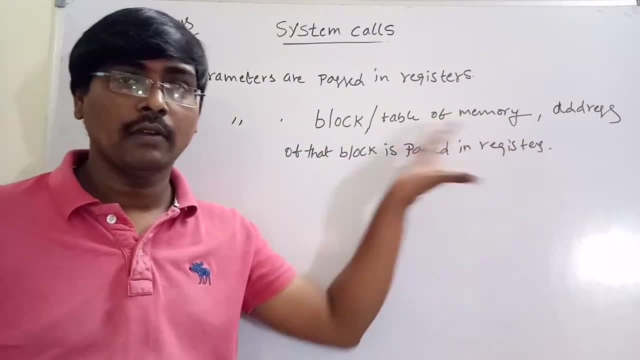 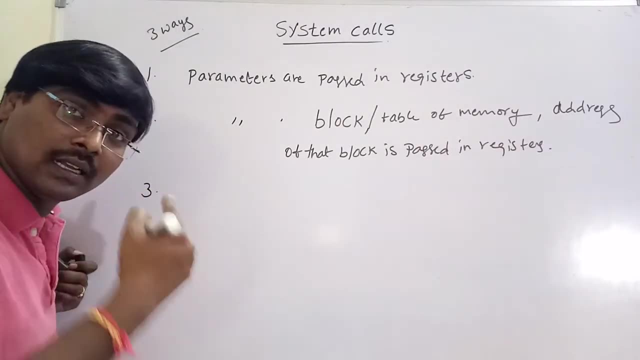 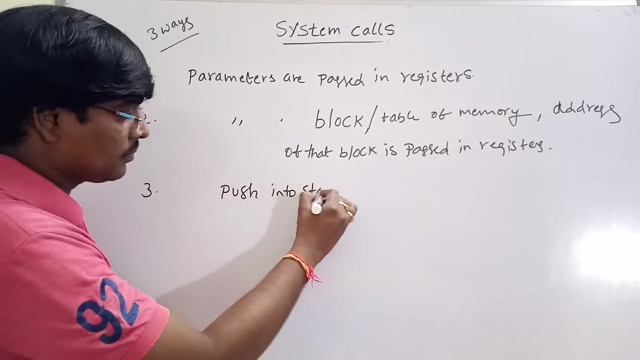 and the address of that block is passed. address of that block is passed in the register. And one more technique is at the user side, that is the programmer side. programmer side: push into the stack. that is, the parameters are pushed into the stack. and at operating, 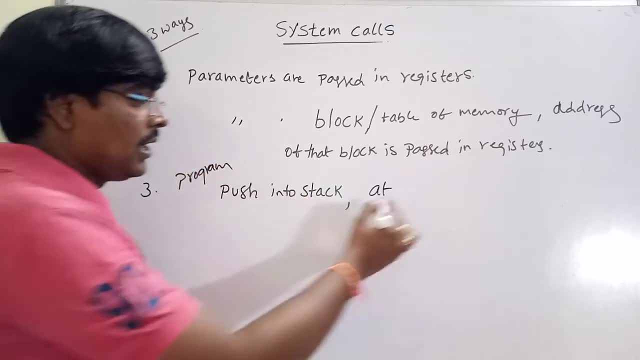 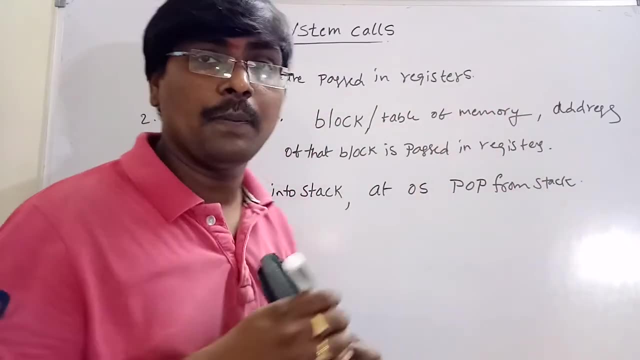 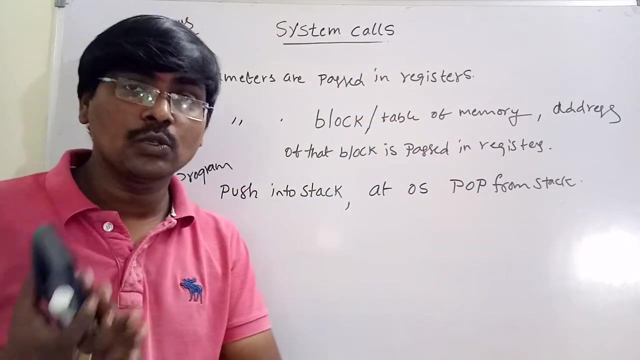 system, which is at programmer side and at operating system, pop from the stack. That is, by using stack, we can pass the parameters. by using stack, we can pass the parameters. These are the three ways to pass the parameters to the operating system. 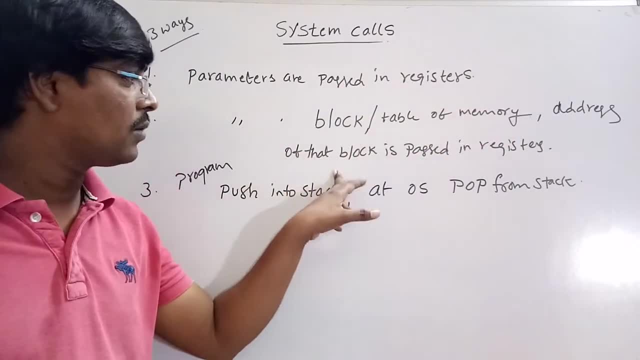 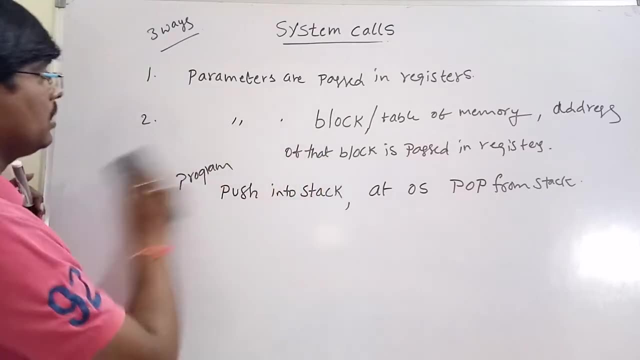 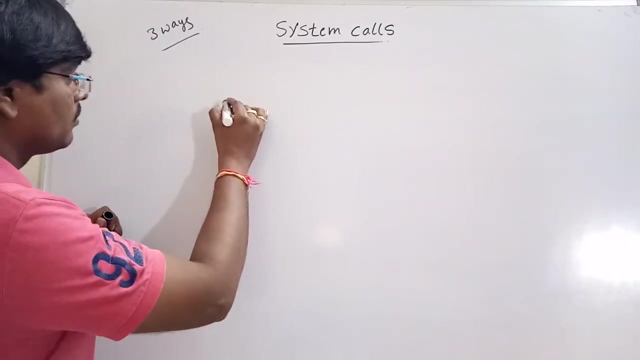 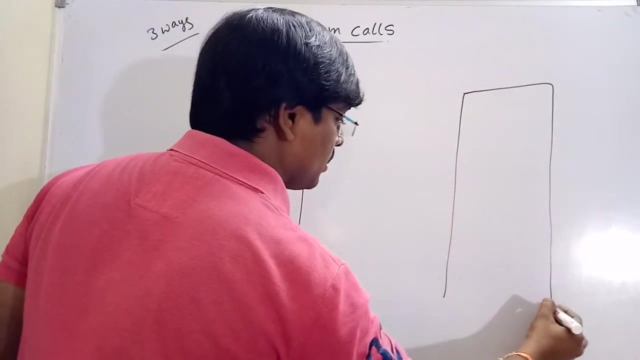 One is directly all the parameters as individual, another one is the address of the entire parameters and another technique is by using stack. So consider a diagram for second one. consider a diagram. Suppose this is user side and this is operating system side. this is user side. this is from. 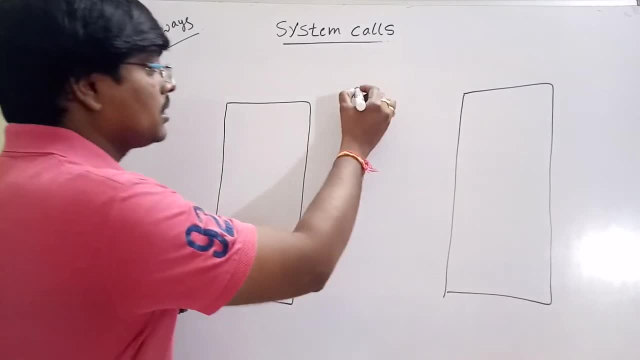 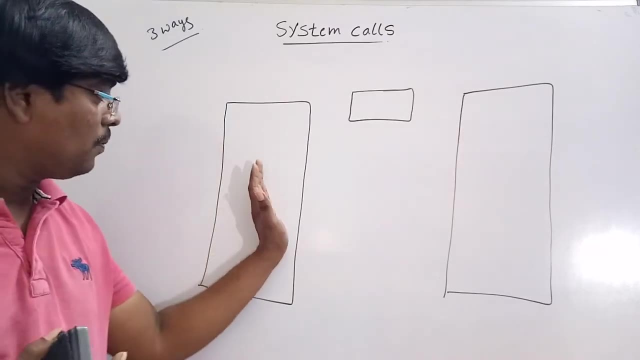 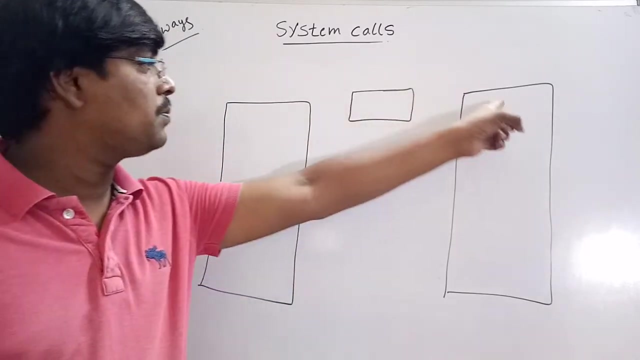 operating system side, for example, assume a register. okay, Now what is the position From the user side? we have to pass the parameters and all the parameters placed on a memory block and the address of that block is passed through the register address of that block. 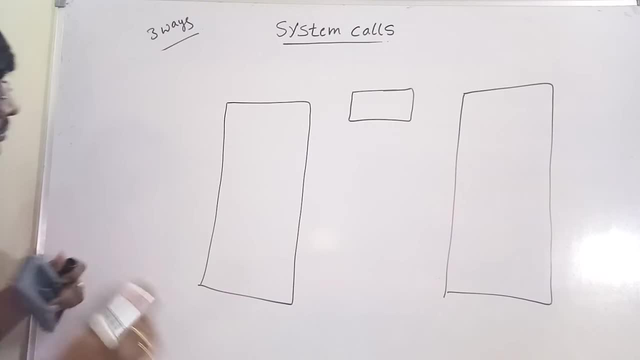 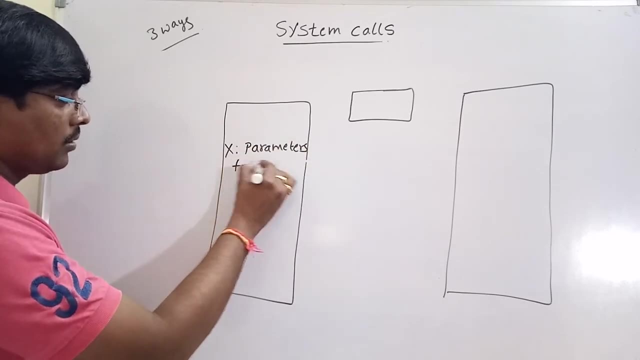 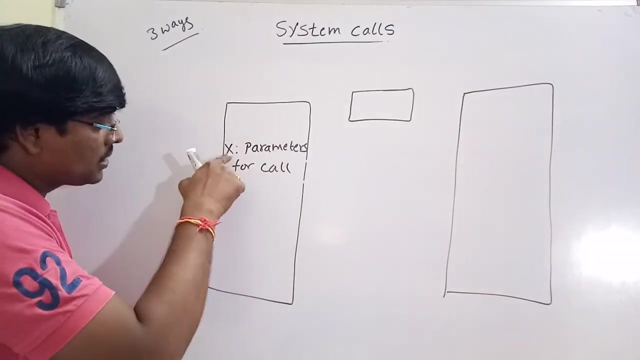 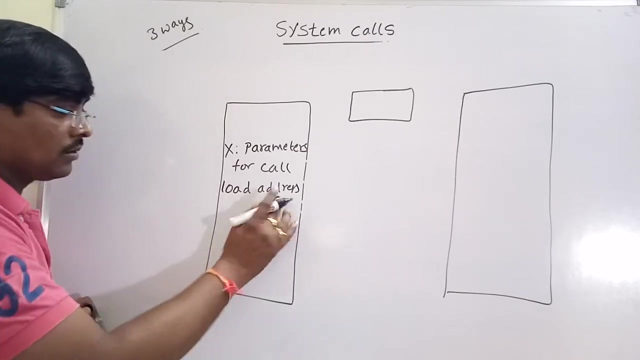 is passed through the register. Okay, For example, x parameters for call, x parameters for call. then what to do? All the parameters are placed. so load address of x, load address of x, for example. here the system call is placed. 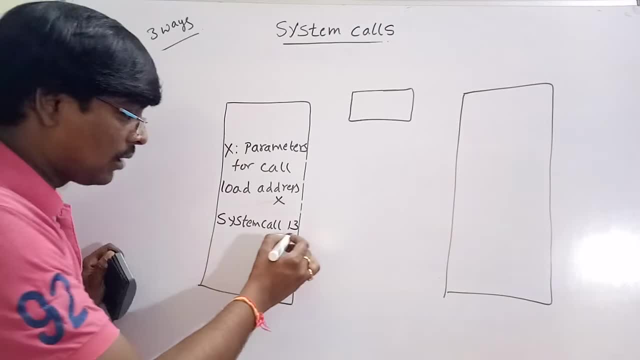 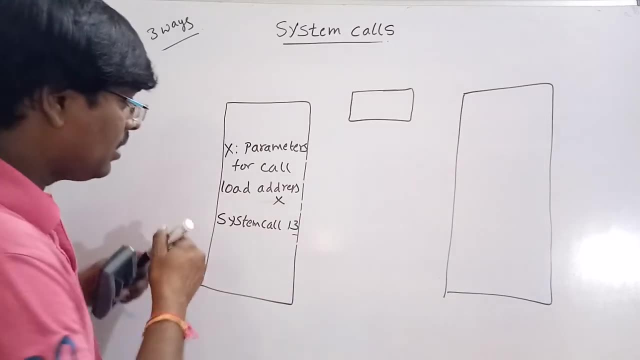 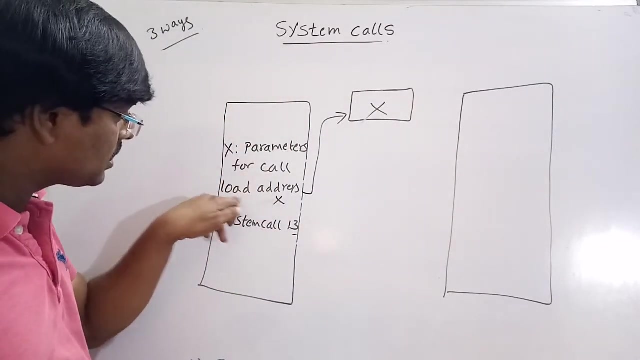 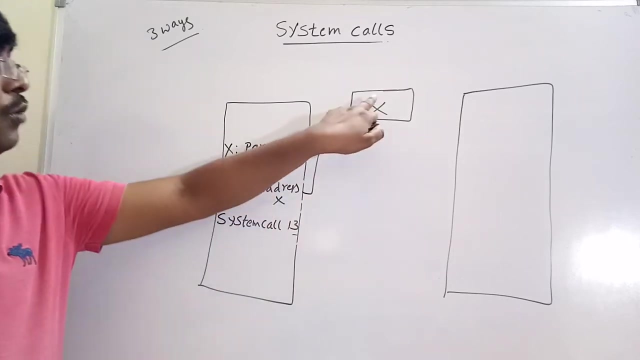 Number 13.. Here not only 13s. Why? because every system call has some number. Every system call has some number. Then here we are, passing in the register. we are passing x, that is, all the parameters are placed at an address x. all the parameters are placed at an address x. so we are passing. 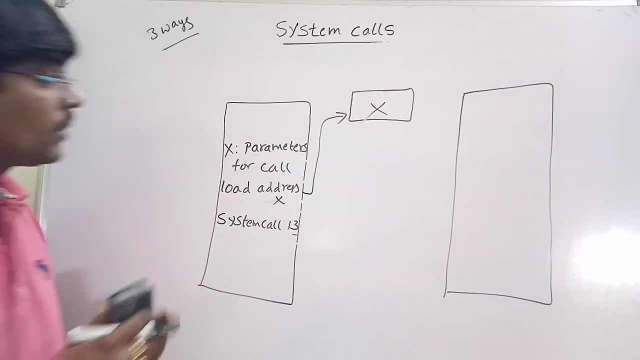 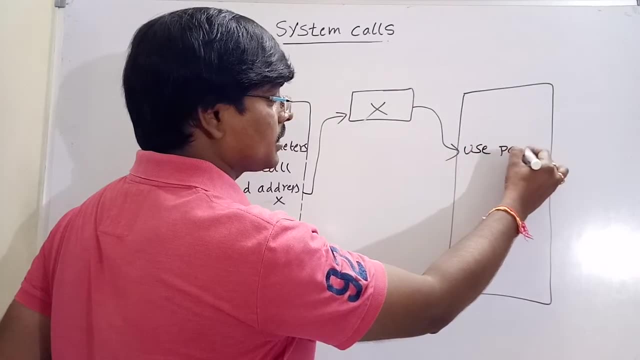 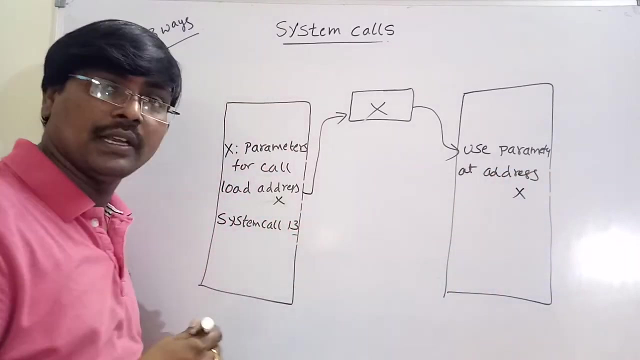 x. We are passing x. Okay, Now for next example. Okay, This is operating system. What the operating system do? Simply use parameters. Use the parameters at address x. Use the parameters that are present at address x. This is the way to pass the parameters. This is system call. 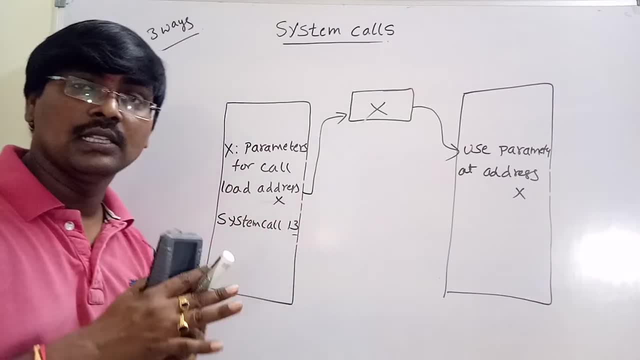 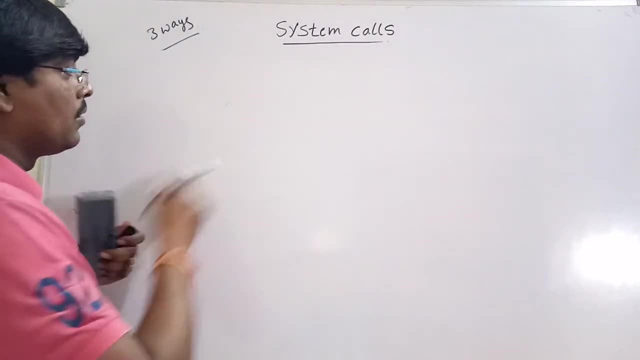 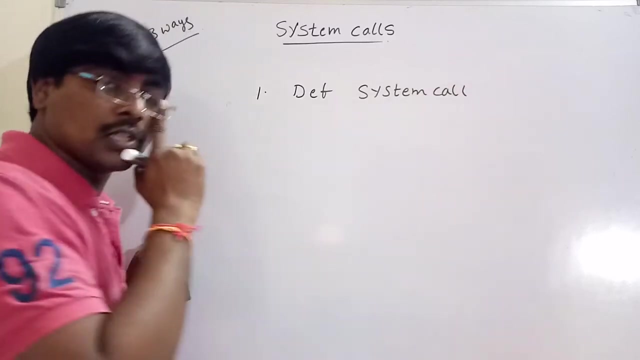 Okay, Once again, what is a system call? System call is simply an interface. Remember, the point is summary. What is the summary? First one is definition of system call. Definition of system call: Okay, Interface between operating system and the process. 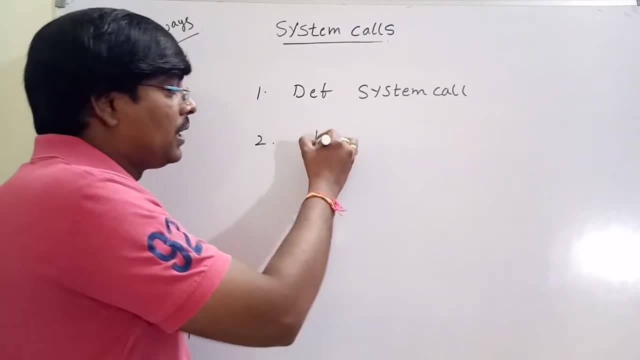 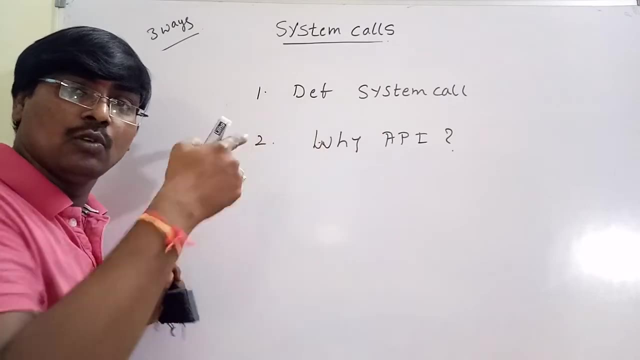 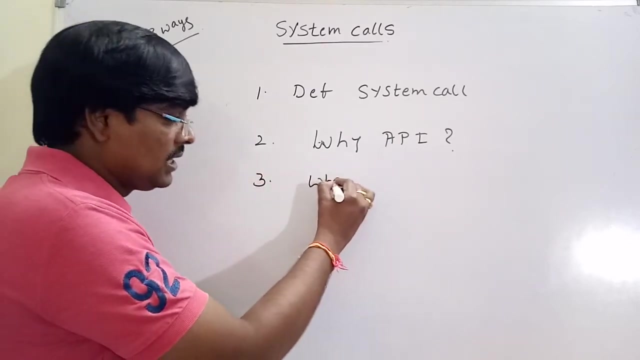 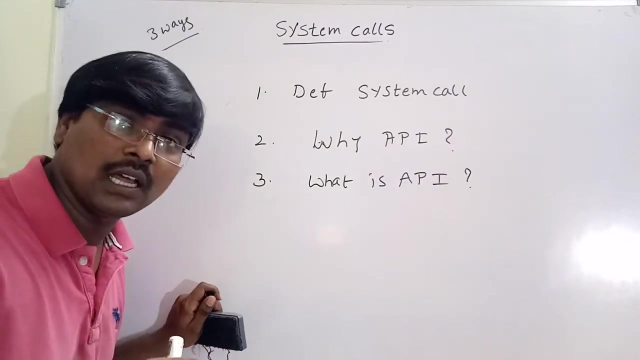 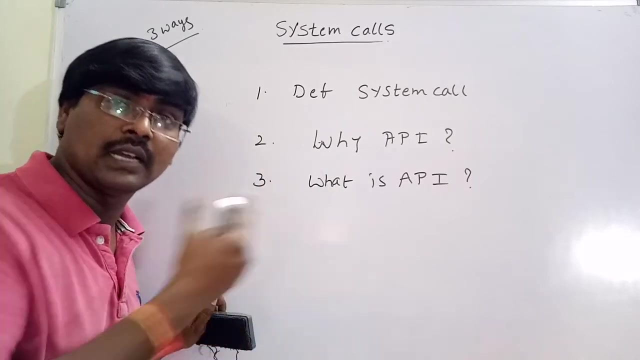 Next one is why we are moving to application programming interface. Why API? Why API? Because a user have to execute many number of system calls for a single program. For that purpose, we are moving API. Next, What is API? API is an application programming interface which contains set of functions, Set of functions that are used by the programmer, And it also includes some parameters and written values. also. Next, How API calls. 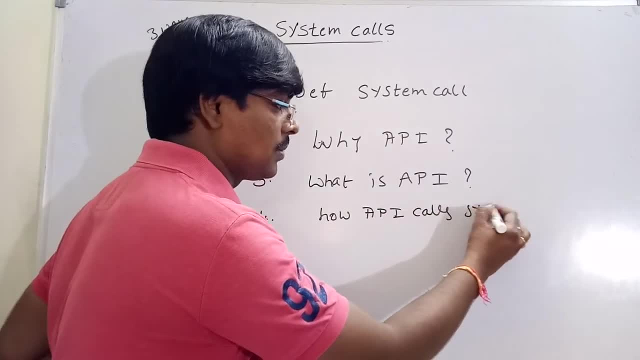 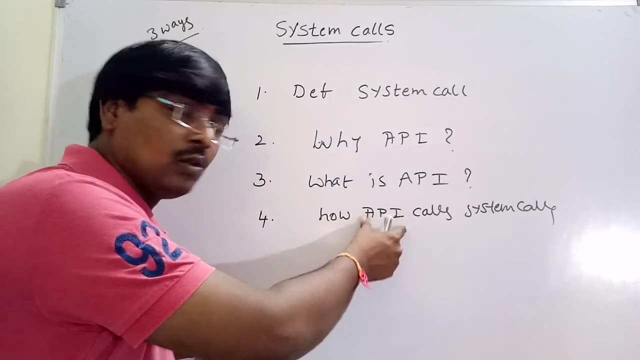 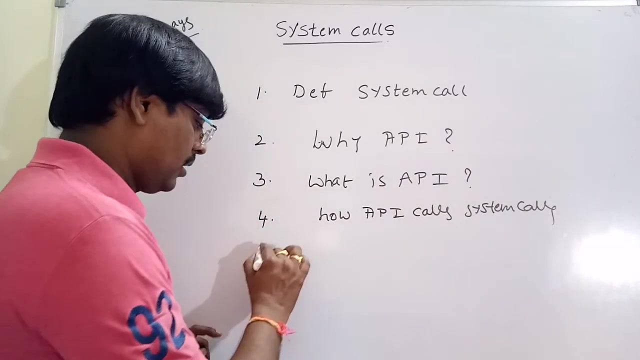 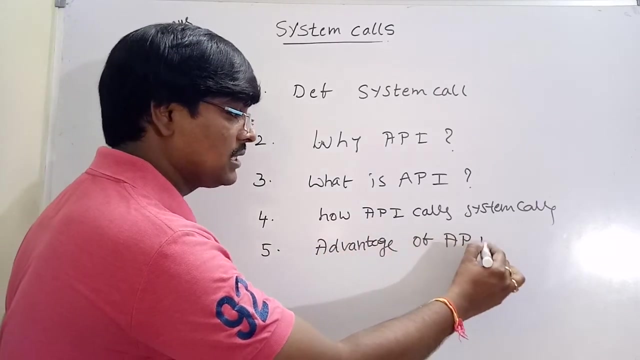